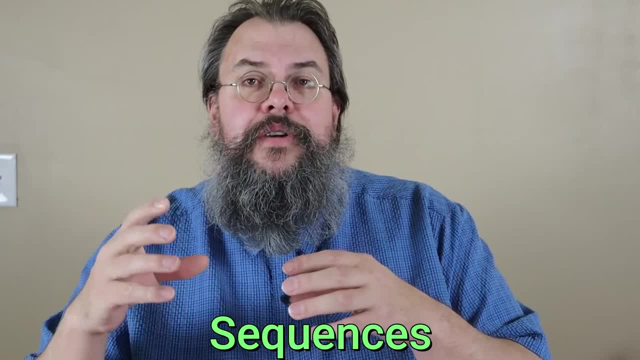 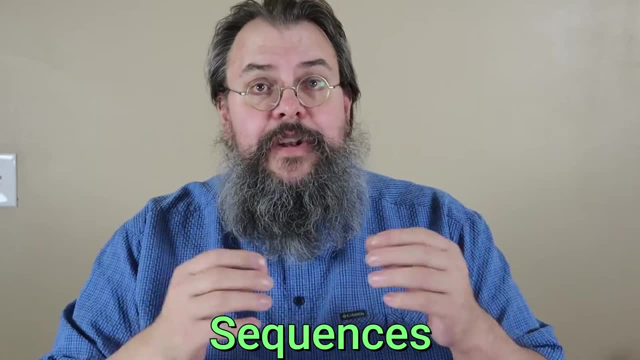 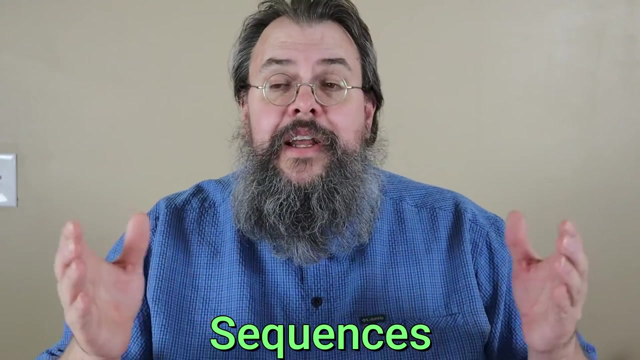 we really want to think of like a list of numbers. So there's like the first number on the list, the second number and so forth and so on, And in particular, we're going to be focusing on infinite sequences. So these are lists which just keep going and going and going. Now, when you say 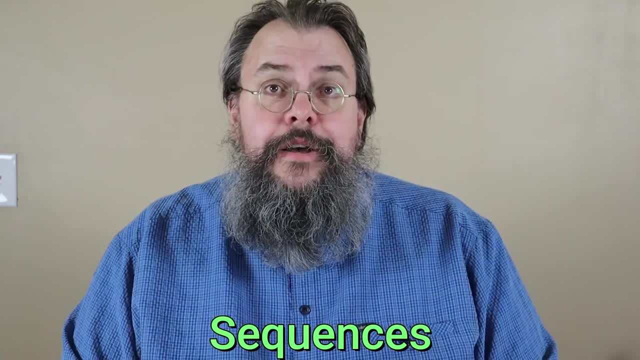 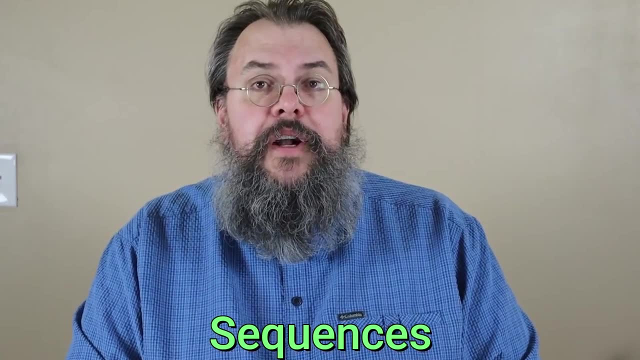 oh, a sequence is a list of numbers. what else is there to say? Well, not really that much, right, It's just. that's what it is. The real question, and where we're going to put most of our energy is saying, hey, what's happening at the end, Because oftentimes we want to say, well, 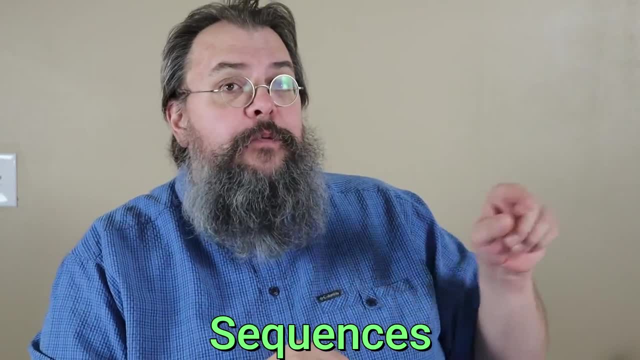 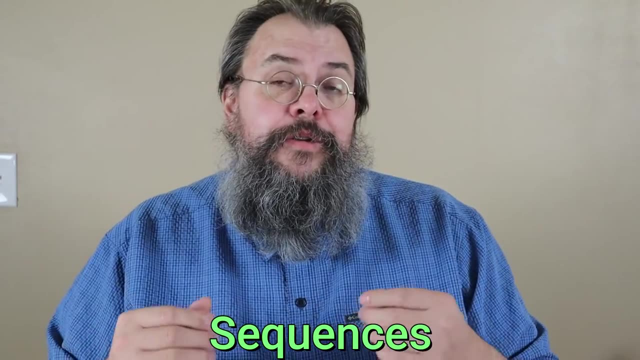 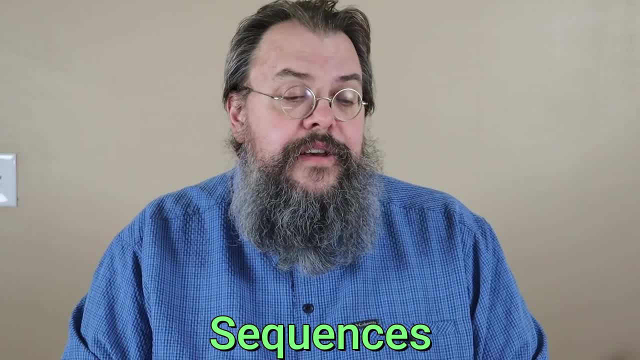 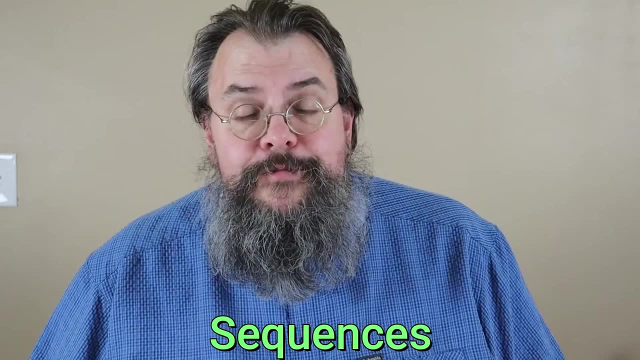 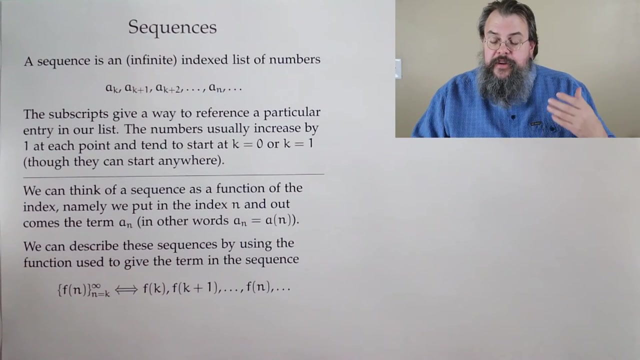 How do we figure out what to say is at the end And what are some tools? That's what we want to talk about today. So let's begin. As we said, a sequence is going to be an usually infinite list of numbers, and they're indexed. And when we talk about being indexed, 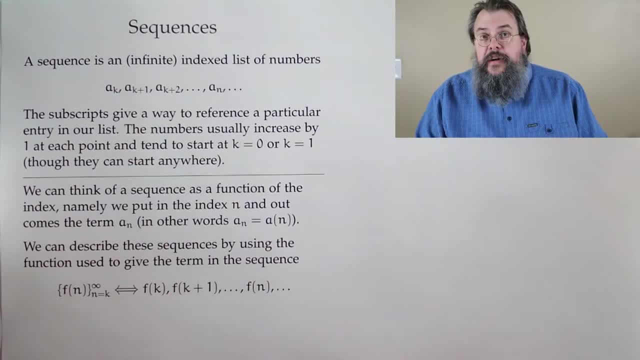 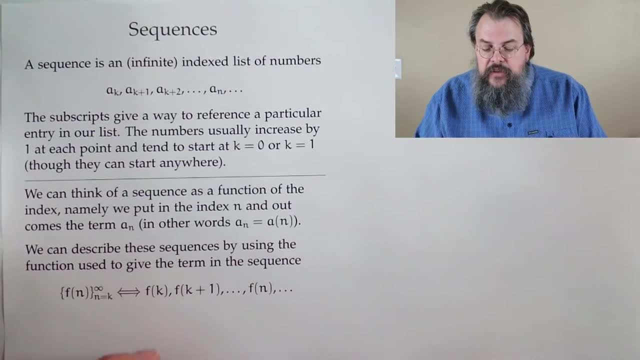 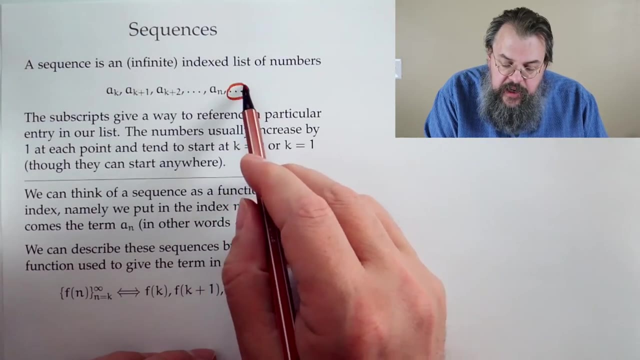 it just means there's a subscript here, So we don't have to start at any particular value, We can start anywhere we want. So the kth one, the k plus first, the k plus second, and so forth and so on, And the dot dot dot. whenever you see dot dot dot, it just means and it continues. 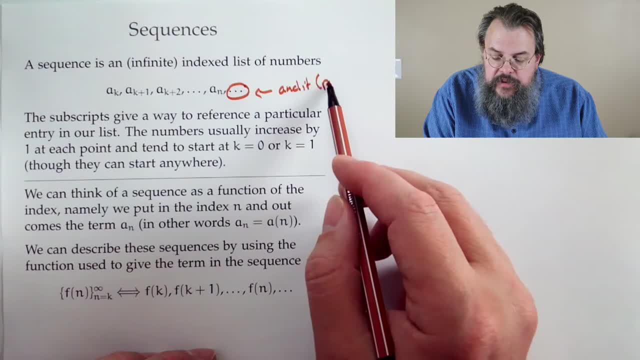 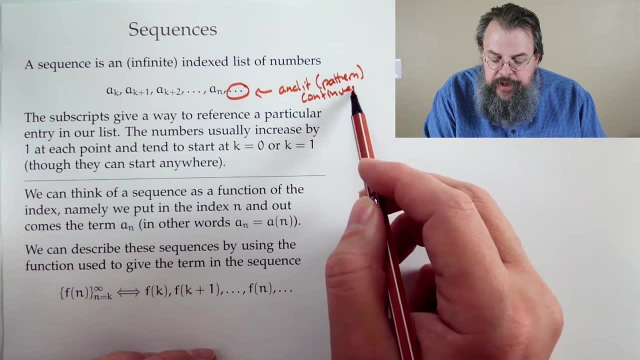 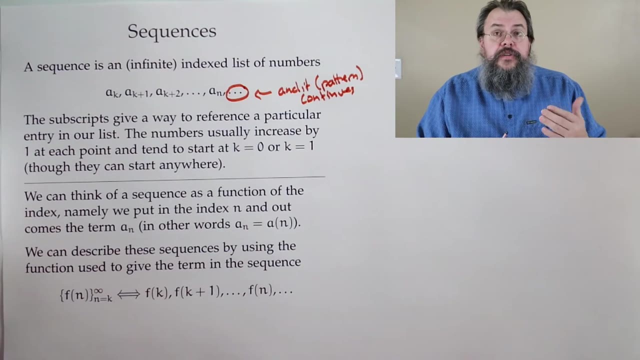 And usually when we say it, we say: there's some pattern here, So there's something that's going to say it keeps going. One of the ways we oftentimes think of these sequences are as functions. We say, okay, we're thinking of where, we input the index in and what comes out is the. 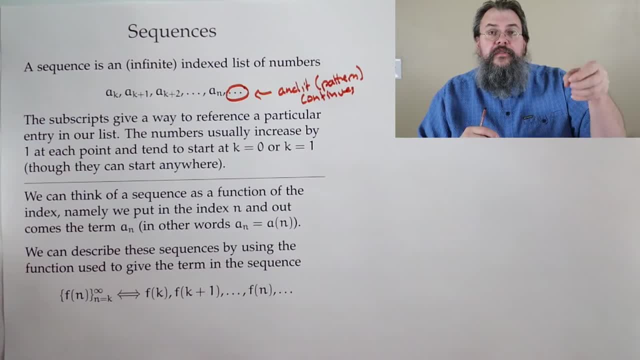 number. that's at that point. So if we put in a five, it says: okay, here's the fifth term in our sequence. If we put in a hundred, okay, here's the hundredth term in our sequence. But of course, 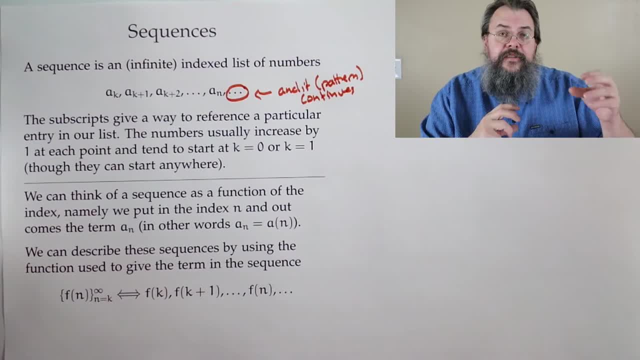 we can also do the opposite, Say, well, here's a function and that can define the sequence. So if I plug five in, that produces the fifth term. If I put a hundred in, that produces the hundredth term. So we'll oftentimes think of sequences in this way as, there being some 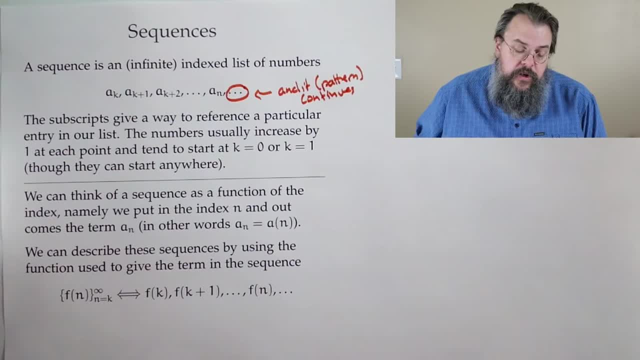 function which helps define them, So we can think of describing it as okay. there's some function which depends on our input, and our input ranges from some starting value, k, up to some ending value, usually infinity. So if you see this notation, 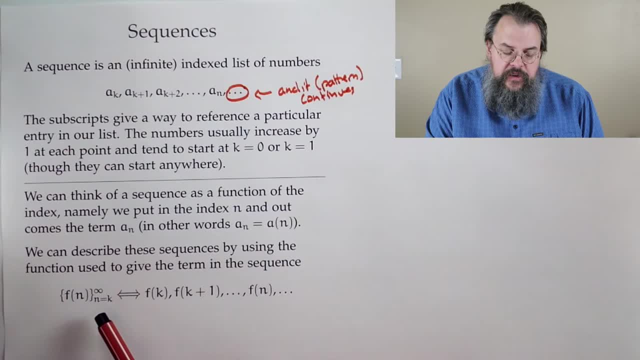 you should think of it as: okay, I'm making a list starting at k and going to infinity, and everything on my list follows this rule. You give me a value for n. that tells me what I should see. That's what I have. Well, what's the big question? The real big question is saying: 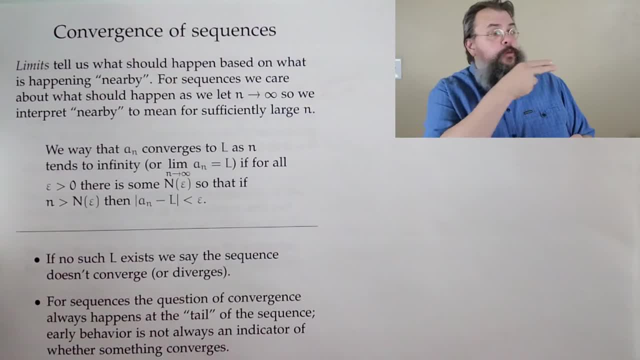 what happens at the end, What's happening way down there as we head off to infinity? The tail- Well, you'll hear that phrase a lot- the tail. Well, we can't pick up our last value, It's just there's not a last one. But maybe we can ask the question: what should the last value be? 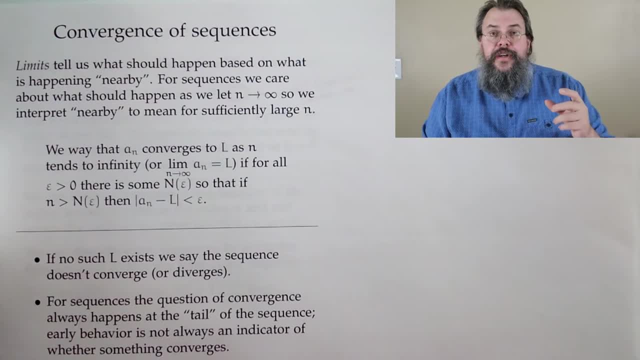 Whenever you start to hear a question which is phrased with a should- well, that really is a limit question. And so we say, okay. well, how do limits work? Well, the idea is we look at what's happening nearby And I say, okay, so I just pick a number close to infinity, like three, right, 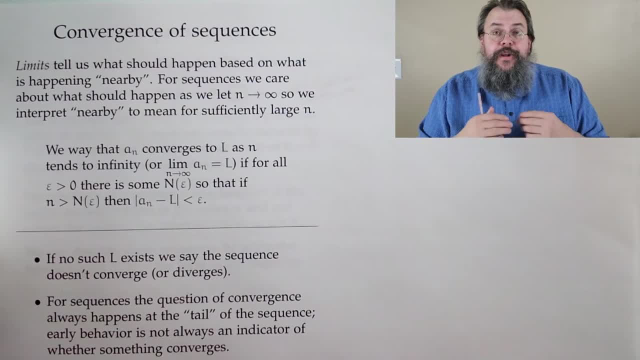 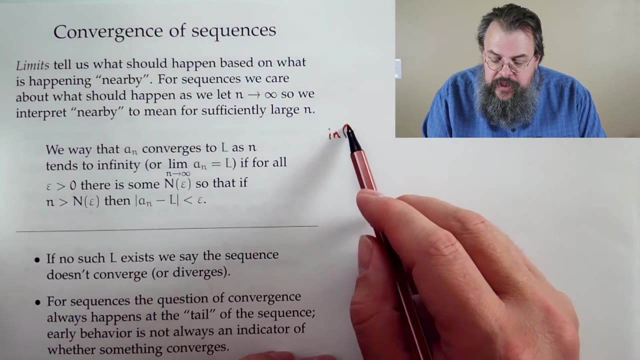 Well, three doesn't feel close to infinity, But, in all honesty, three is as close as any other number. So what do we mean by being close? Well, when we think of infinity, if you think of the word infinity, you can think of it as being what? Well, it really has two pieces You can think of. 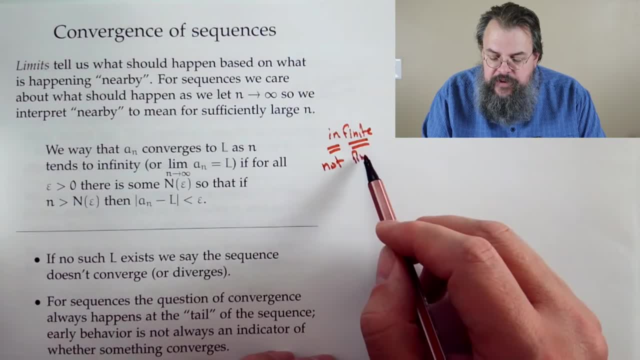 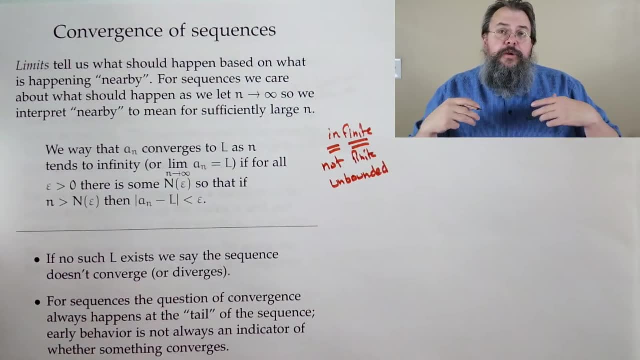 it as not and five, So it's not finite, or a better way to think of it, is unbounded. So when we talk about going to infinity, it means we're getting bigger and bigger and bigger. That's what we mean when we talk about going to infinity. 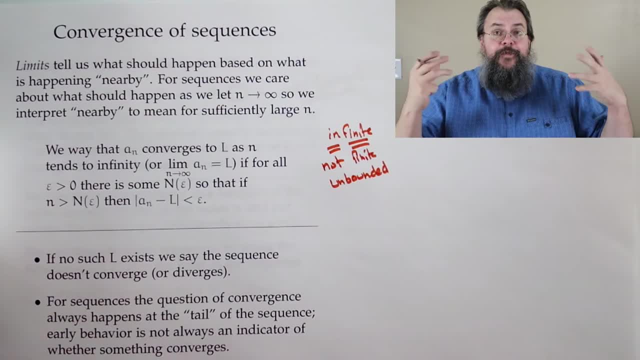 So close to infinity just says sufficiently large values. So now we're ready to talk about the formal definition of limits. Don't get too nervous, We're not going to use the formal definition very much, but just for the record it's there. 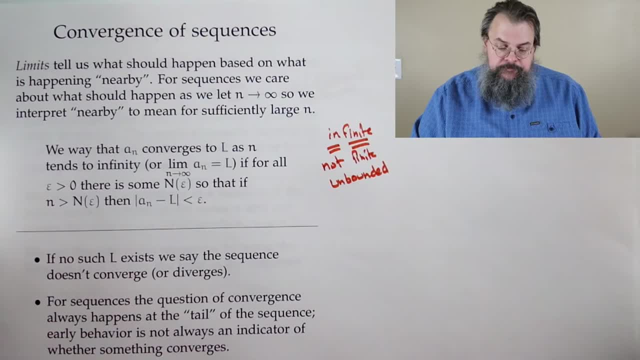 if we ever need to refer to it. So our sequence: A sub n converges to L as n tends to infinity. In other words, the limit as n goes to infinity of A sub n is L if, for all epsilon greater than zero, there's some big number, n, which depends on epsilon. 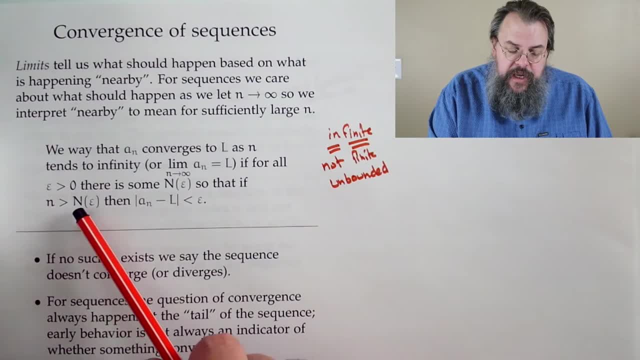 So that if we're sufficient, So that if we're sufficient, If we're sufficiently large, so this is that big number n which depends on epsilon- says how far do you have to go, Like, how far down do you have to go, for say okay, from here on out. 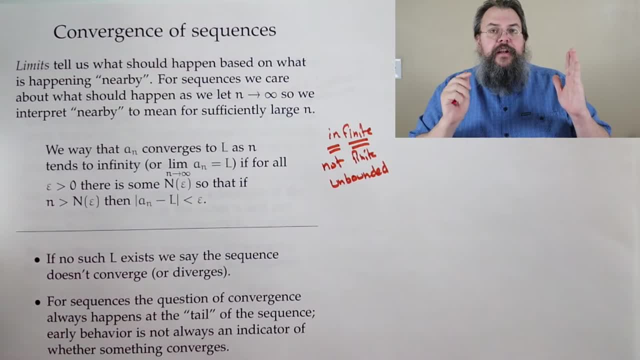 So if I have an n, epsilon says: okay, from this point on, the first part doesn't work, but from this point on ever after, we're always close to L within epsilon. That's the conclusion. Now you might notice that. wait a second. I thought limits had epsilons and deltas. 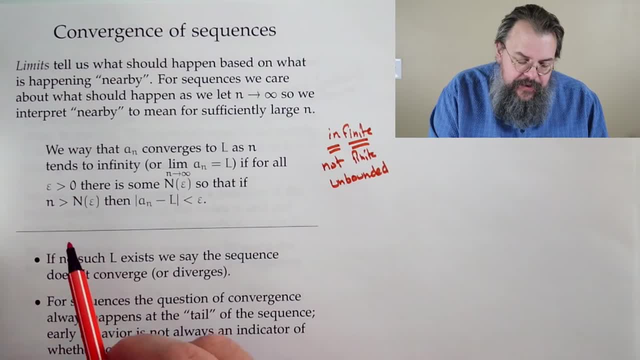 Where's the delta? And the answer is: this is sort of acting as the delta. So when we think about delta, delta is a measurement of closeness, So we're close to something. So here our closeness is being close to infinity. 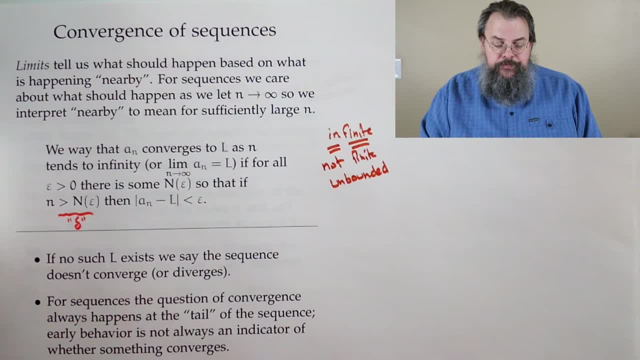 And we're doing that by saying: oh, you're sufficiently far away. It is possible that there is no such channel. You can come up with sequences that do that. in fact, it's pretty simple to do things like, for example, 1, minus 1, 1, minus 1, 1, minus 1, and so forth. 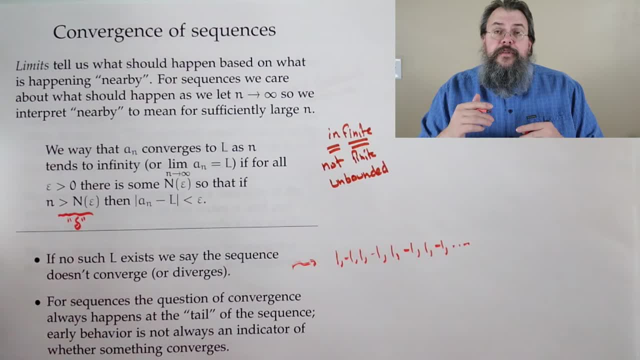 That's a very simple sequence to describe. And what happens? Well, you just keep jumping: 1, minus 1, 1, minus 1, 1, minus 1, 2, 2, 2,, 2,, 2, 2.. 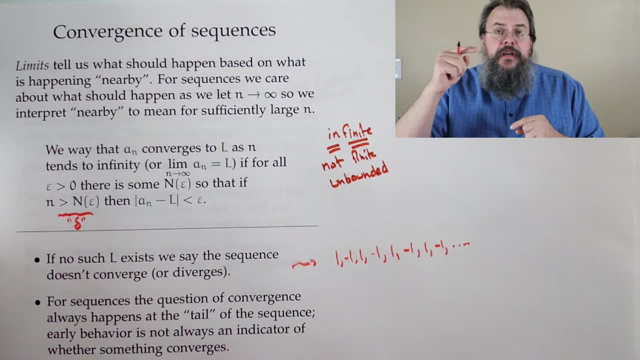 The problem is: what do I get close to? Well, do I get close to 1?? Well, half the time, yeah, but half the time I get close to minus 1.. And the thing is there's a gap and I can't be simultaneously close at the same time. 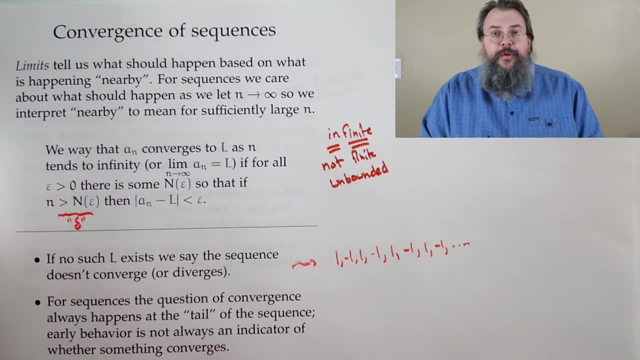 So this is an example Which doesn't converge. Now you might say, well, wait, maybe I converge to 0.. No, no, no, no, not in our class, that's not how we think of things. There are people who sort of say, well, what if that? 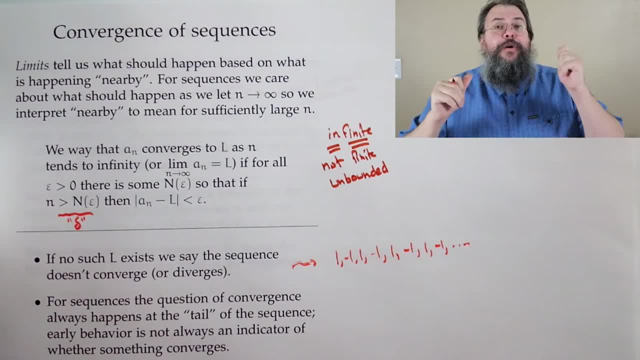 What does it mean to do that? But no, no, if we converge, we have to converge to one number, one and only one behavior. Now there's other things that can happen. For example, you could have 1, minus 2, 3, minus 4, 5, minus 6, and so forth. 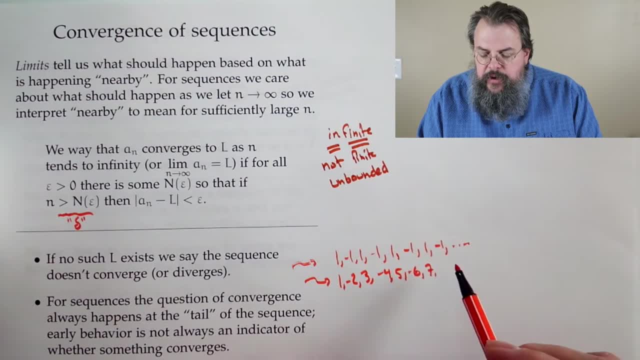 And so on, So where you change the sign at every stage, but you also get bigger. So you're going doom, doom, doom and you're wildly going back and forth. Okay, forget it, hopeless, hopeless, not going to happen. 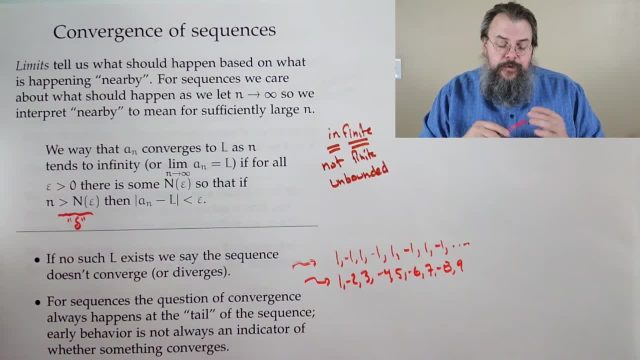 All right. so the question, of course: where do things converge? That's what we're after, and we've already said it, but look, it says it here again: Focus on the tail, Don't be enticed by the tail. 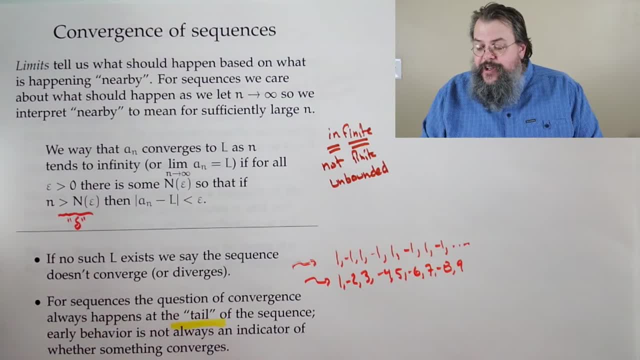 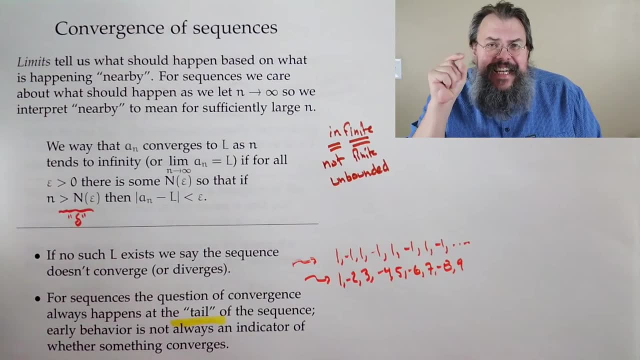 Focus on the tail. That's basically the first couple of terms. It's easy to create sequences where the first few terms are just so. so teeny, teeny, tiny numbers. They're basically like specks of dust. They're so small you couldn't even see them if you pulled out your microscope. 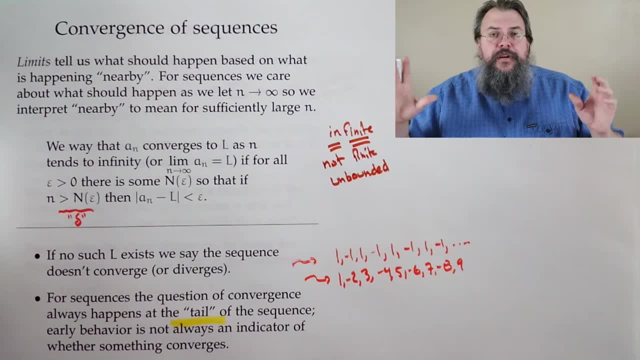 And even for the first million, billion, trillion, however many terms, we can make sequences which are just like: wow, look at that so tiny, but we're not interested in the start, It's the end. down there, way down there, like way, way down there. 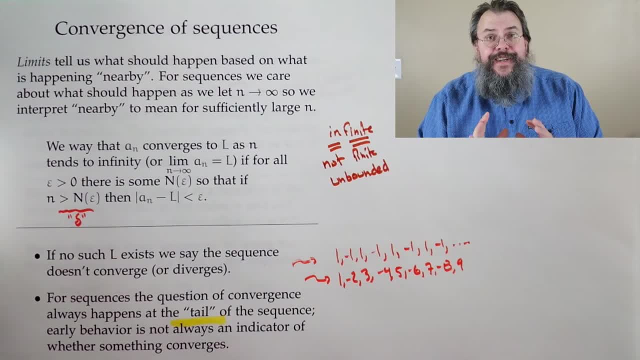 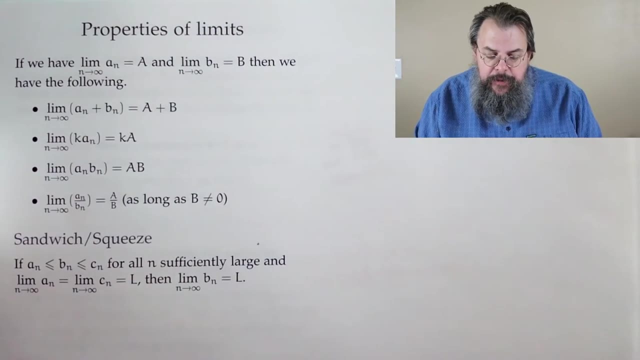 That's what we're interested in. So don't be tempted by what happens at the start. Focus on what happens at the end. That's the real question. so pay attention. So what are some basic properties? Well, we have the same properties of limits that we always have. 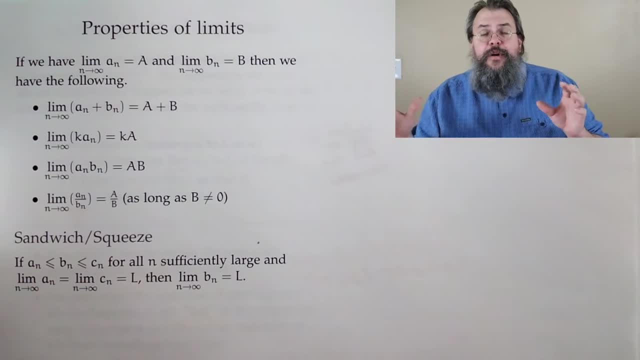 These should feel familiar. We should be like, wow, aren't these the properties of limits we had before? And the answer is yes, it's exactly the properties of limits that we had before. And things which seem intuitively obvious turn out to be true. 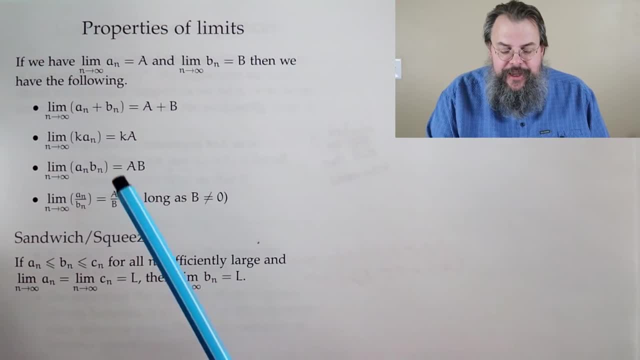 Sometimes the word intuitively obvious does not mean easy to prove. Things such as: hey, if the limit of one sequence goes to A, the limit of the other sequence goes to B, and if I add the two sequences together, producing a new sequence? well, 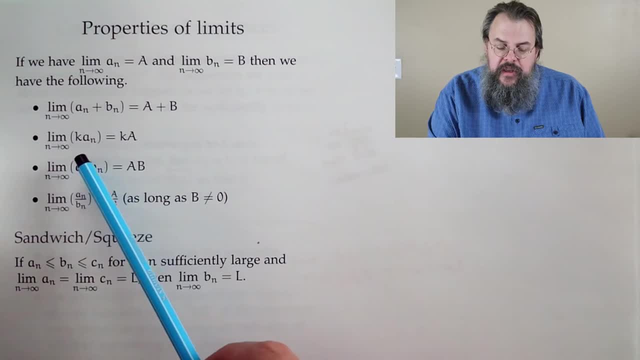 that goes to A plus B. If I scale a sequence, then that goes to the scaled value of whatever it goes to. If I multiply, then that goes to the product. And I can even divide, as long as what I'm dividing by is not zero. 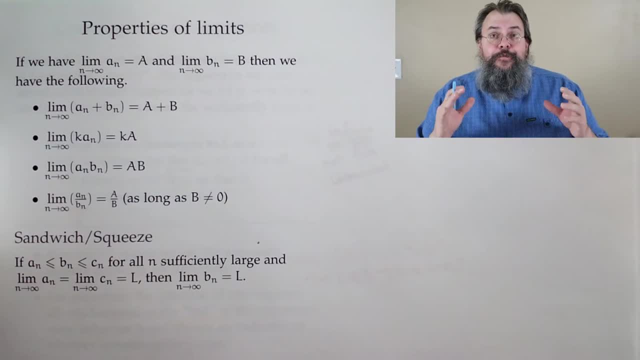 Now, if what I am dividing by is zero, well, more work, more work. And then, of course, we can start to talk about the squeezing. Okay, what is that? Well, it says: look, suppose you have some sequences and you have three of them: A, n. 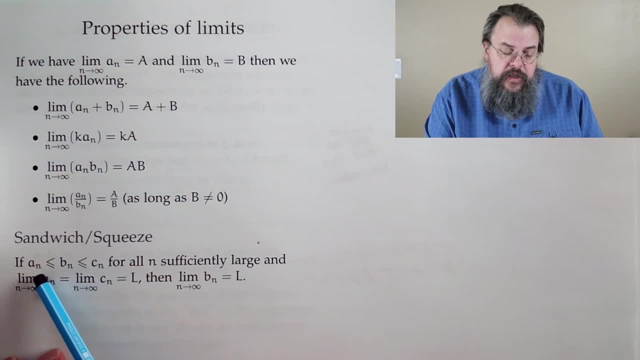 B? n and C? n And B? n is in between, sandwiched between A? n and C? n, And as you head off to infinity, A sub n gets close to L, because that's what the limit is: C sub n gets close to L. So you're saying, look, A sub n is getting close to L in some 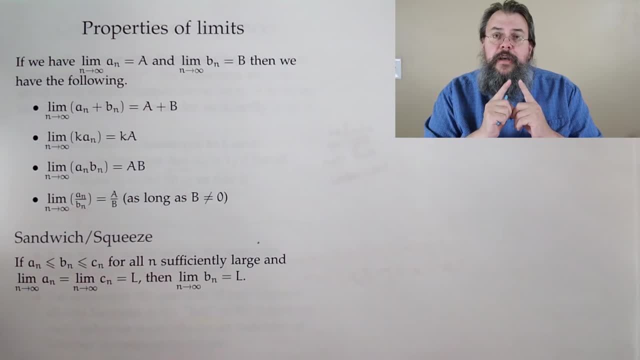 way. And then C sub n is getting close to L. What's true? Well, the thing in the middle also has to get close to L. Okay, so true, The same principles, No big surprises. Great, We love it when there's no big surprises. 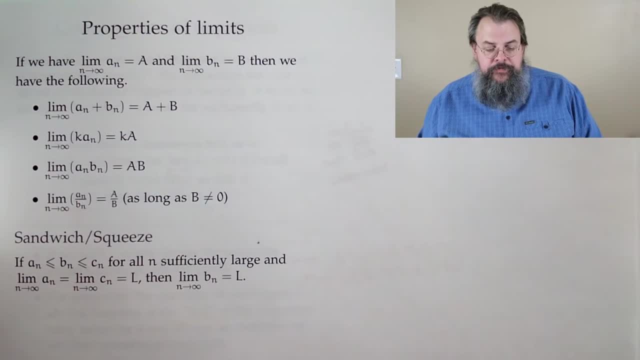 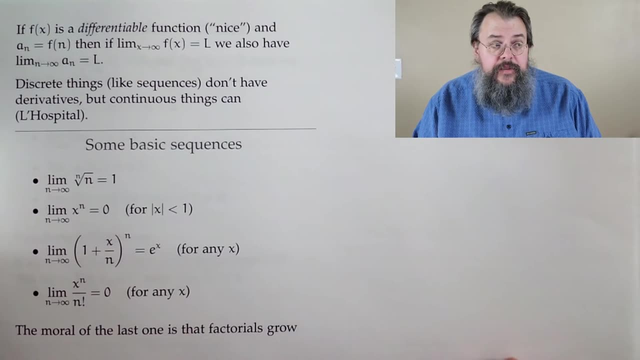 It makes it easier for us to figure out what's going on. Now suppose we have a function f of x And we're thinking of it as a function defined for all numbers, And let's say it's a nice function differentiable. 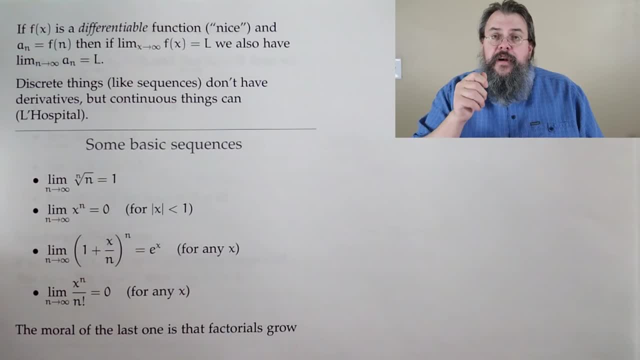 And we look and say we can create a sequence by looking at the function, at integer values. Our conclusion says, hey, if the function as a continuous function goes to L, then the place where we look at the integer values also goes to L. 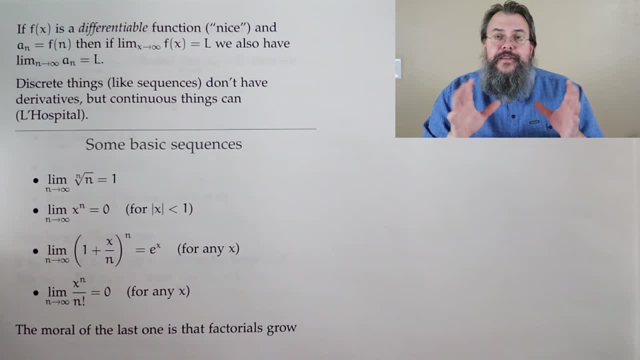 And we're like, great, wow, Isn't that trivial? Wait, why isn't this completely obvious? Why do we need to actually say this kind of thing out loud? There is some subtlety here, And I want to make sure that we understand the distinction. 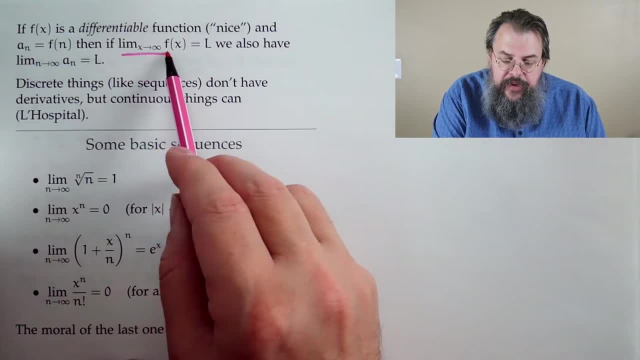 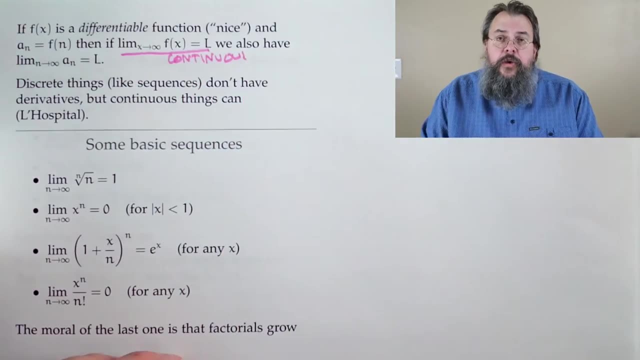 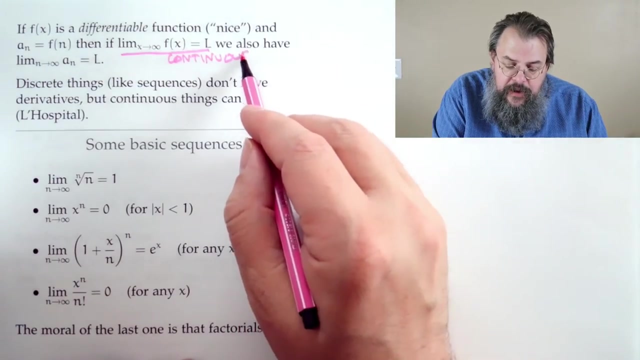 So when we write the limit as x goes to infinity, f of x equals L, we're in what we would call the continuous setting. And that is: Look, we have all the points, We're not skipping anything. So we take all the values along the way. 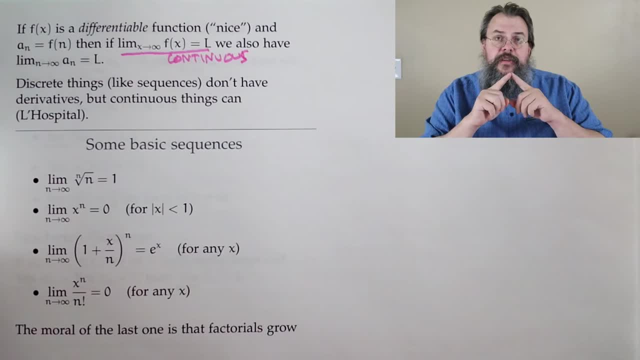 So when you talk about the continuous, that's the continuum, when we think of the continuum as the line. But what about the other part? Well, when we're talking about this limit, as n goes to infinity, of a sub n equaling. 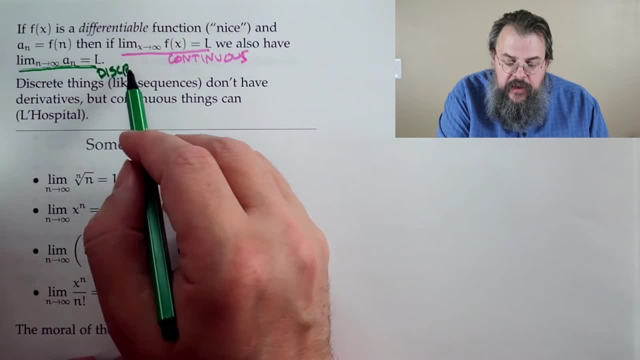 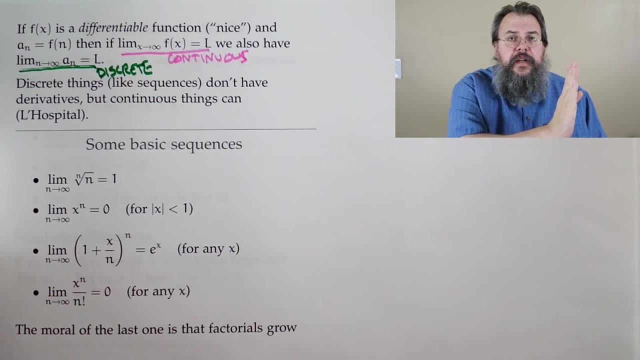 L, that's in the discrete setting. And here it says: Look, we're not looking at every single value, We're sampling at the integers. So what happens at 3, at 4, at 5,, at 6, and so forth and so on? 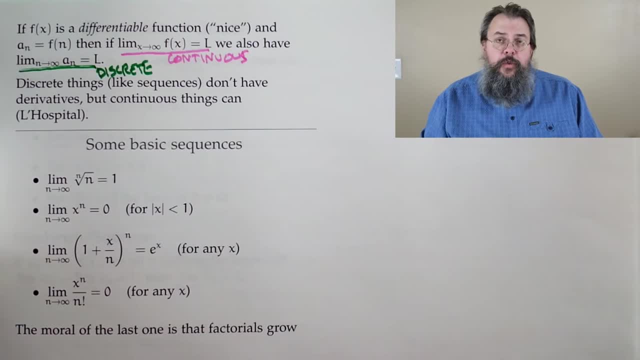 Now, where's the difference between them? Well, the thing is, whenever you sample, you're sort of losing the behavior of what's in between, And so there's a uh Okay. So If you look at the picture, well, we might have a curve. 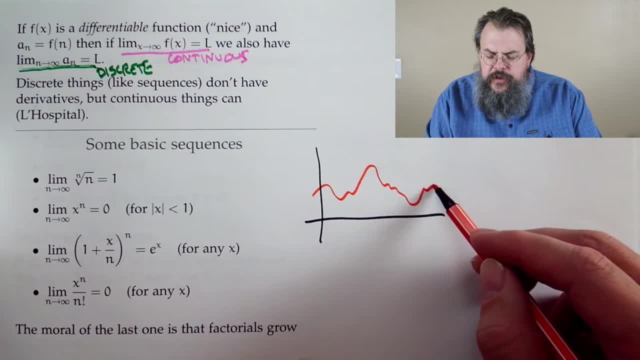 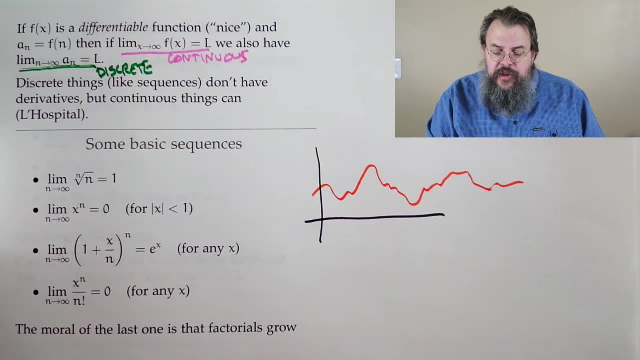 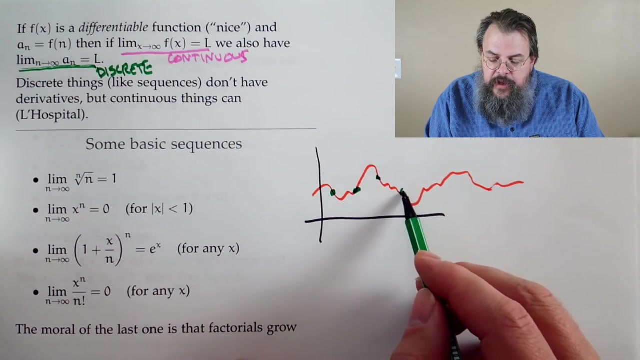 And so as a function it could be doing some rather unusual things, Going up and down, doing all sorts of crazy stuff. But when we start to sample, we only are looking at the curve at certain points, And so it might seem a little bit less erratic. 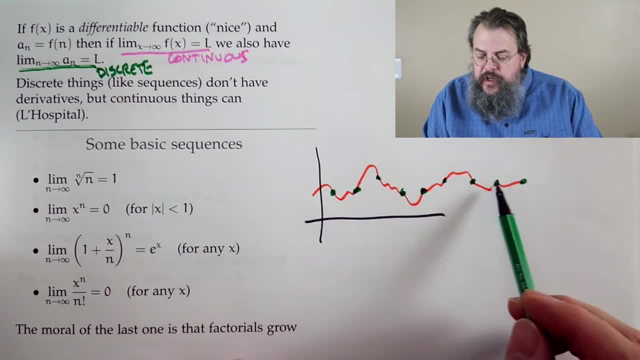 And all of a sudden, our, our function says: wow, samples, it's looking pretty good, But the function, ah, in between it's all sorts of craziness goes on. So there are subtleties, So be careful. 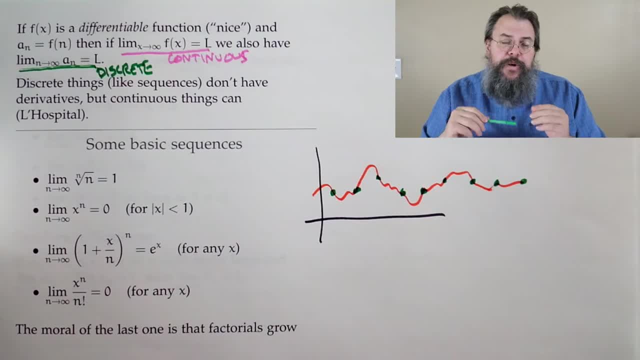 Don't take things for granted. But when our functions are nice and we say, okay, they're behaving nicely between the points, so we can talk about the limits, then we say, great, We can use our continuous tools. What's an example of a continuous tool? 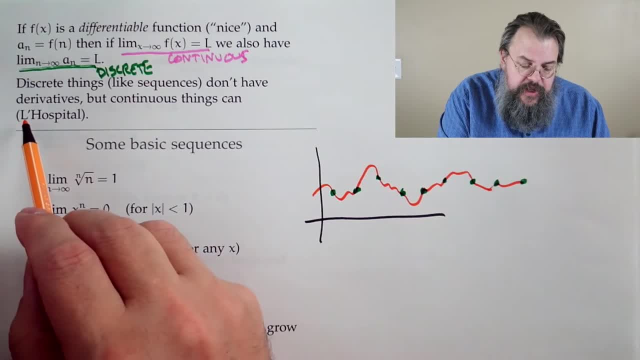 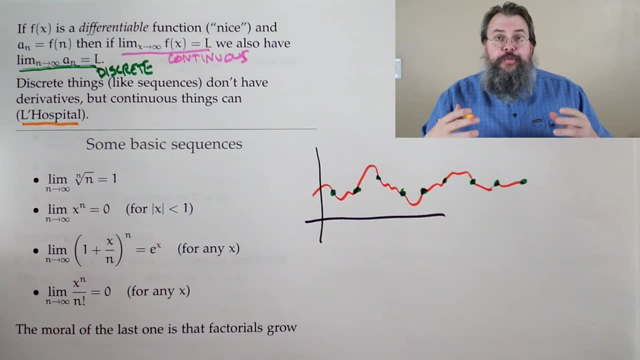 Well, one of our favorite examples is, uh, L'Hôpital, L'Hôpital. Now, of course, why do we like L'Hôpital? Because we can do things like go, ho, ho, ho, L'Hôpital, ho ho, ho. yeah, that's a lot. 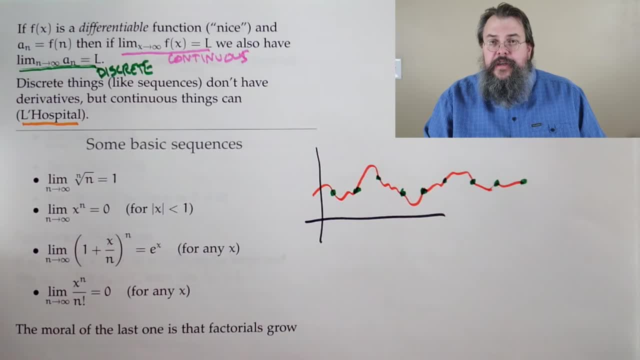 of fun to do that, But it's also a wonderful way to handle various things like like limits, And now we can use this to look at some basic sequences. So the following- these aren't just random, All these are important as we go forward. 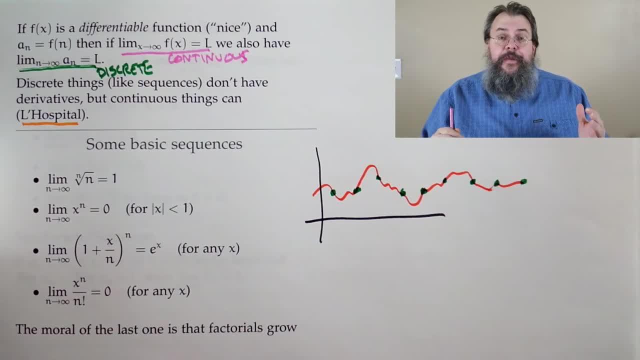 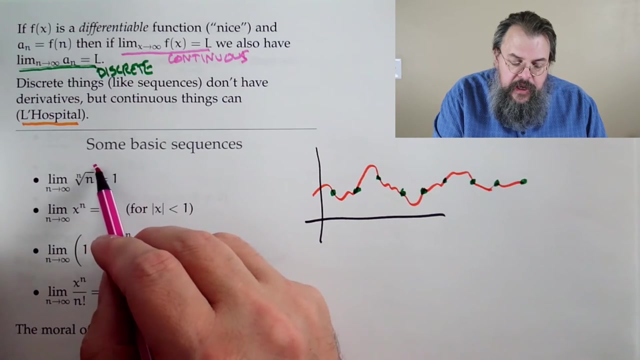 So let's take a few minutes and talk about them. So limit as n goes to infinity. of the nth root of n, The claim is that's one. Well, what's going on? Another way to write the nth root of n is this: is really n to the power 1 over n? 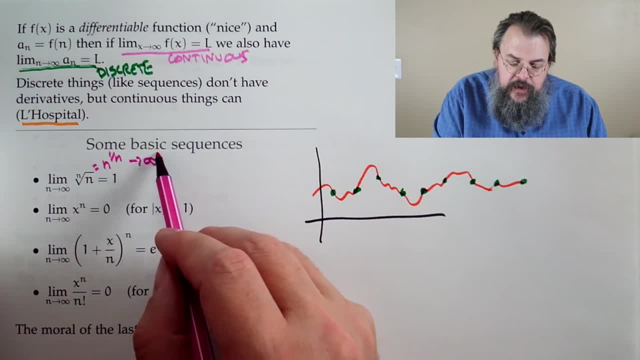 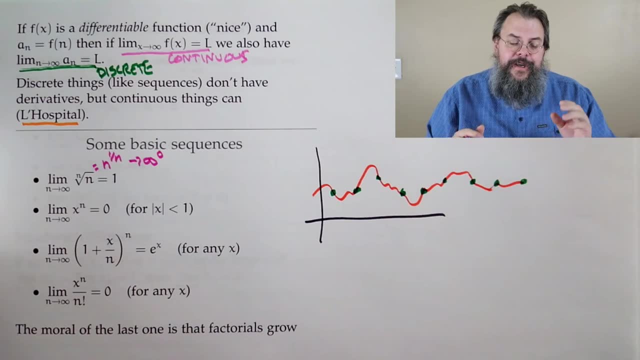 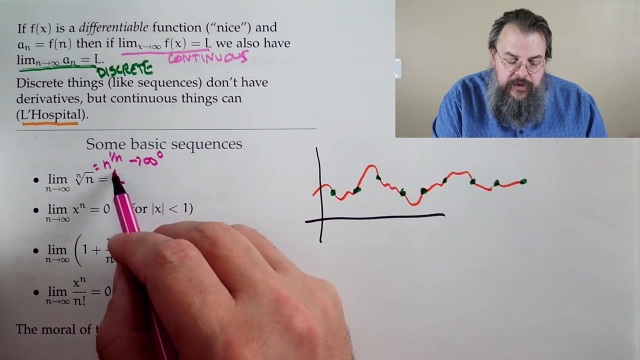 And what's that doing? Well, it's going to infinity, to the zero, And infinity to the zero is more, More, More, More work, more work. okay, well, for a second, let's, let's just call our limit L, so we say, okay, our limit is L. well, now what we want? to bring that exponent down, because 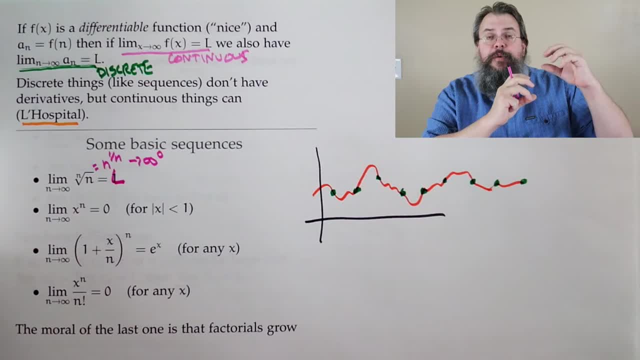 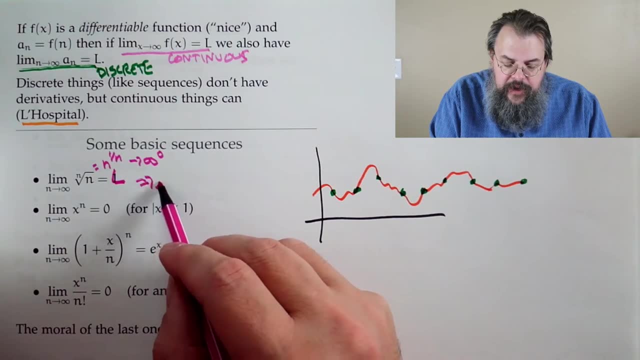 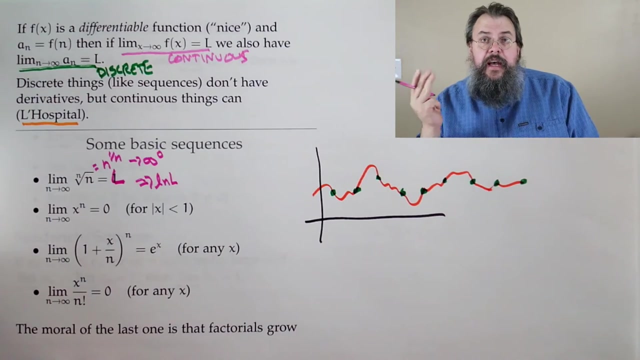 we can't really handle something to the something. but we could do fine with products. so we could say: look the log of L. and now we can pass log through limit, because log is a continuous function. limits can come in and out of continuous functions. that's a nice thing about continuous functions, that's our. 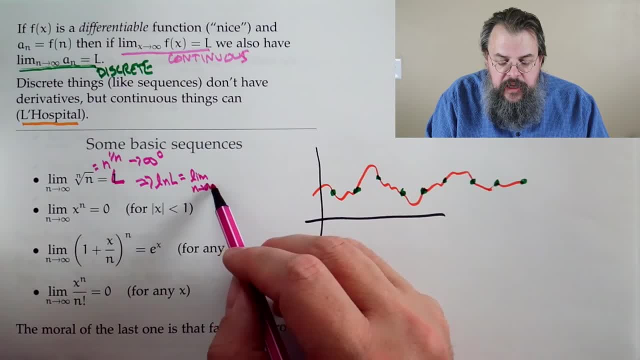 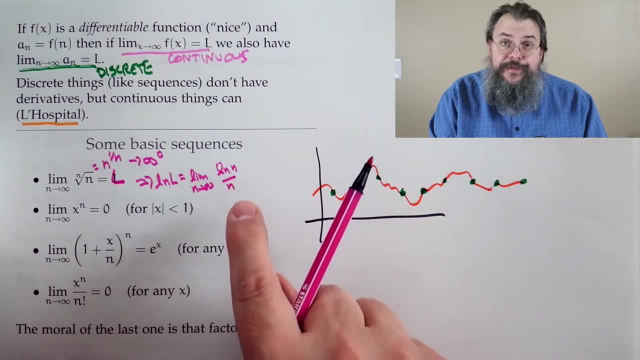 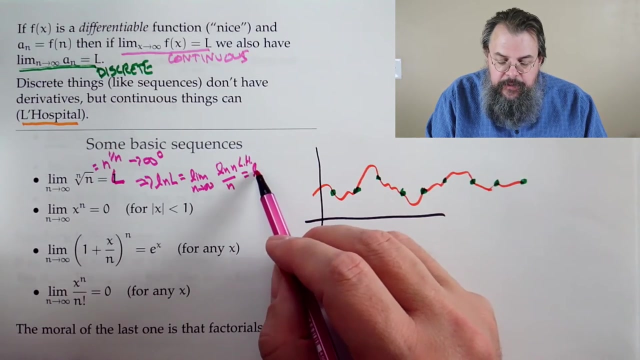 limit, as n goes to infinity. and when I take the log here, that's going to come log of n over n. well, that goes to infinity, over infinity. great, do let hope be down. low, bit down, mon ami. that goes to the limit, as n goes to infinity. and 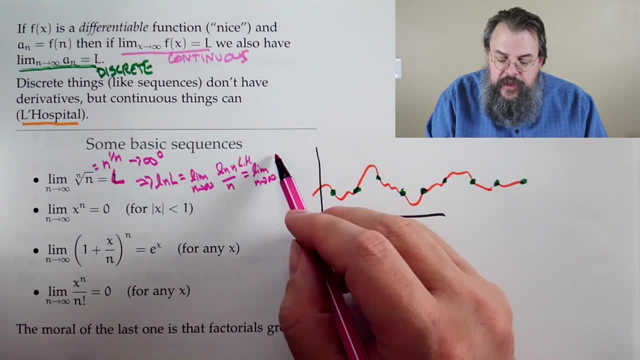 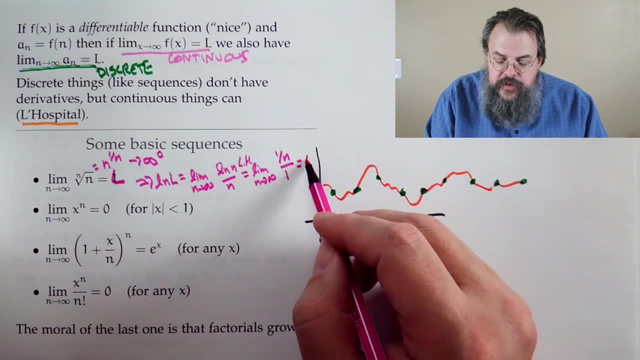 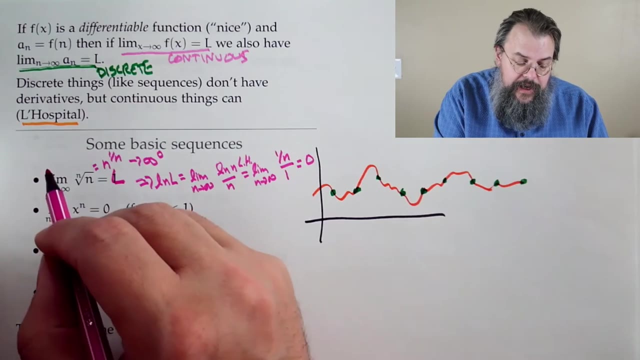 now I'm thinking of n as the variable, thinking here as the continuous, so I can take things like derivatives, one over n to the one which goes to zero. Oh great, so the log of our limit is zero and therefore, aha, it is, as we claimed, one. 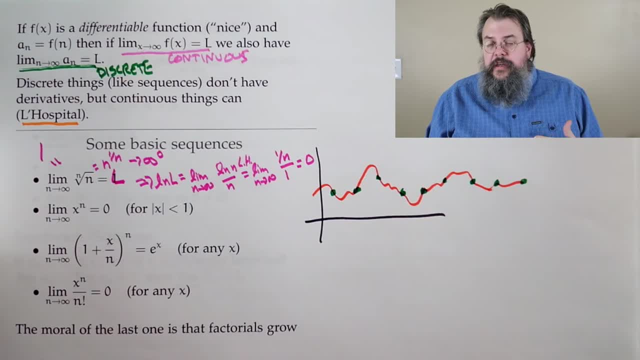 All right, how about x to the n? Well, x to the n, it depends on the size of x. because what does x to the n mean? It means that at every stage we multiply, so it gets bigger and bigger, and bigger if our x is large. 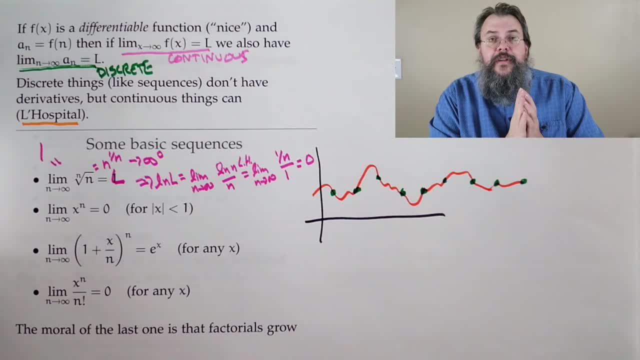 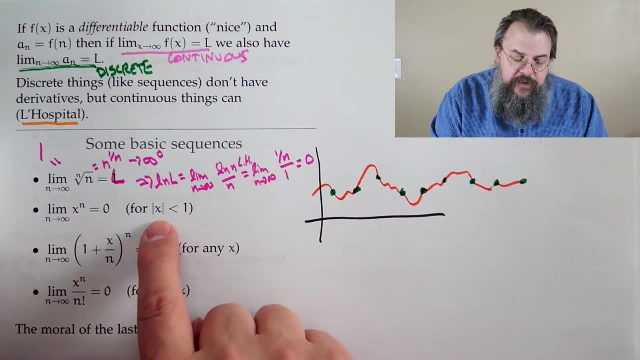 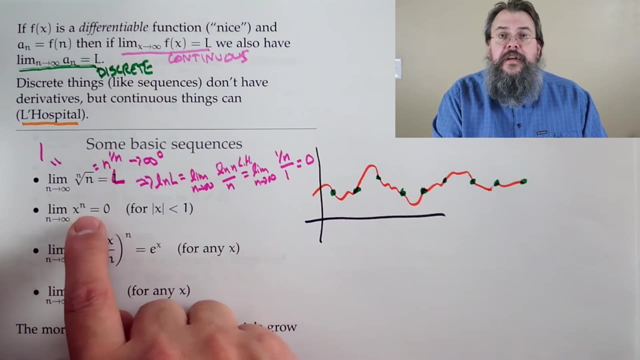 On the other hand, it gets smaller and smaller and smaller. if our x is small- and the important one is if the size of x is less than one, so the absolute value is really think of it as size. if our size is small and we raise it to a large power, 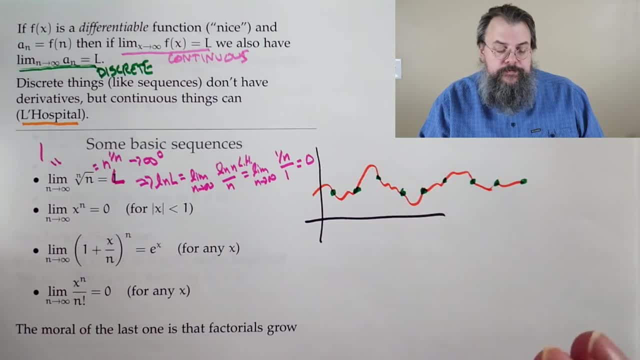 it goes to zero. it goes to zero, All right, good. Now how about this one? One plus x over n to the power n Claim is it's e to the x. Doesn't matter what your choice is for x. 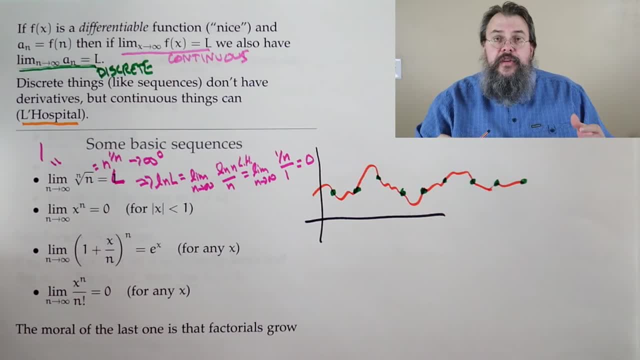 you could choose: x equals one, x equals minus one, x equals 100, it goes to e, to the x. How do you do it? Same procedure here. Say: look, take the log, because it's going to one to the infinity. 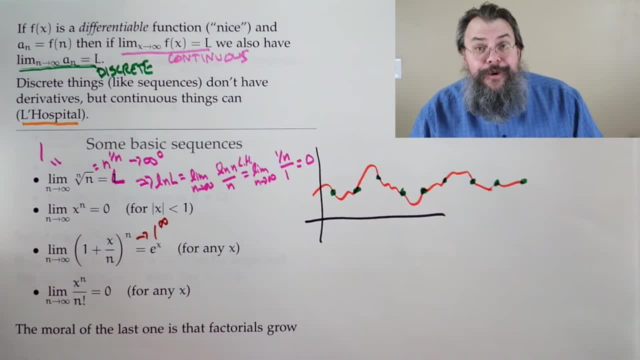 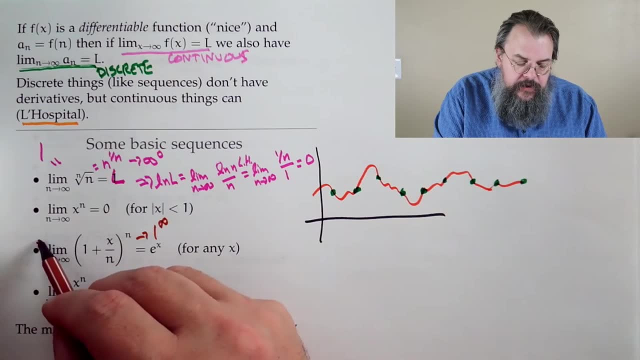 All right. Well, what is that? More work, That's what one to the infinity is. So if you take a log and let's, we'll call this l again for limit, We could say: look, the log of l is. 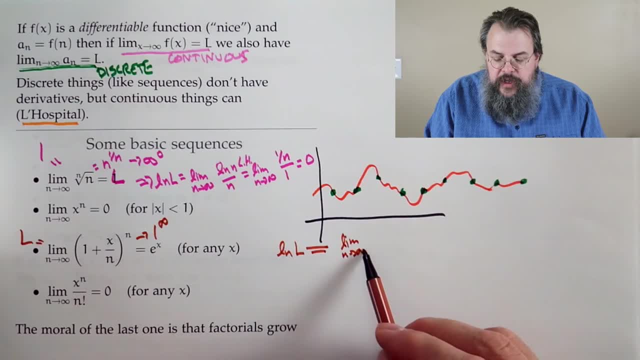 and it's the limit, as n goes to infinity. We bring this way down, So it would come down in front and we're going to push it all the way downstairs. So one over n. natural log of one plus x over n. 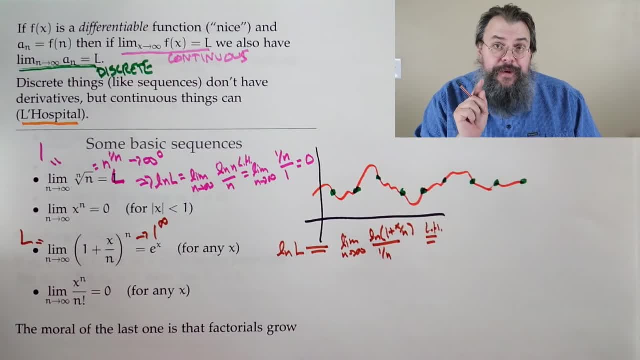 Now taking L'Hopital. This one, pay attention. n is going to infinity, So we're going to think of n as the variable x is just some constant, So that's treated like a number. So you always want to keep track. 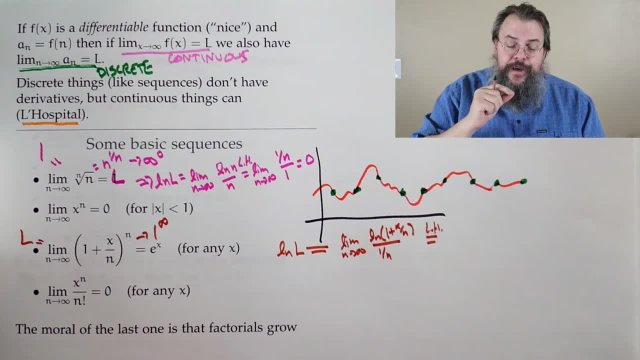 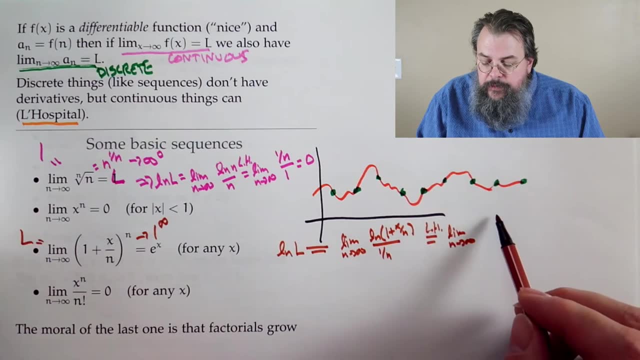 What am I taking rid of with respect to what do I treat like a number? What do I treat like a variable? So this becomes the limit, as n goes to infinity, of one over one, plus x over n times, minus x over n squared. 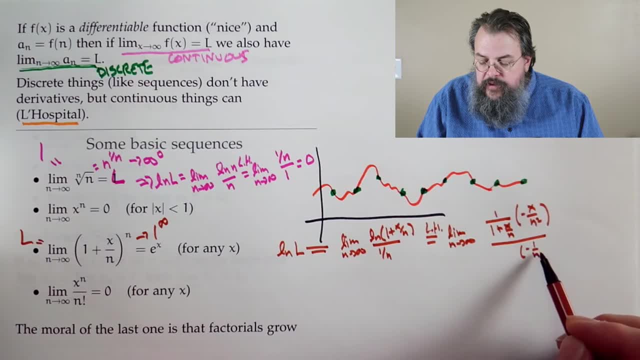 That's the root of the top with respect to n, And negative one over n squared. That's the root of the bottom with respect to n. And then we're like, whoa, this is nice. The negatives cancel, The n squareds cancel. 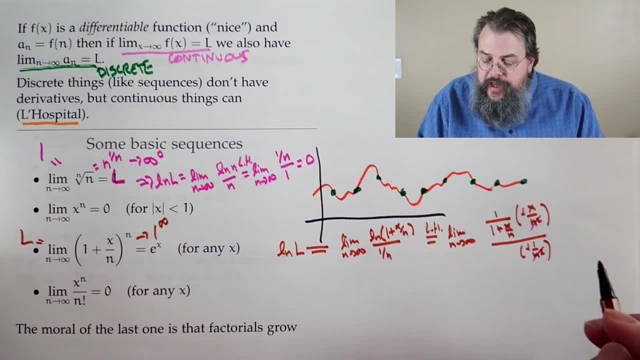 The x over n goes to zero, And so our answer is x. That's the log of. our limit is x And therefore our limit is e to the x. In some sense you can actually say: this is how e to the x is defined. 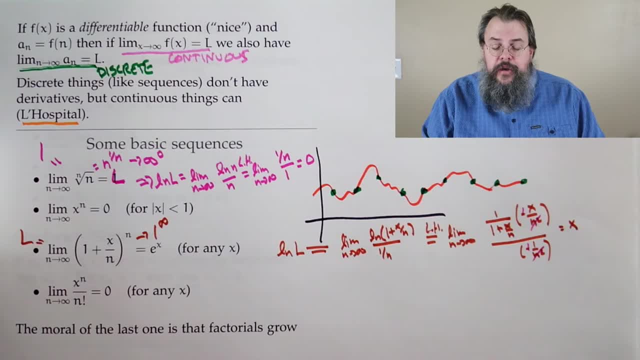 e to the x is defined to be this limit, And then you can explore. well, what does that tell you about the behavior of e to the x? Now the next one, really very important idea: What's the limit as n goes to infinity? 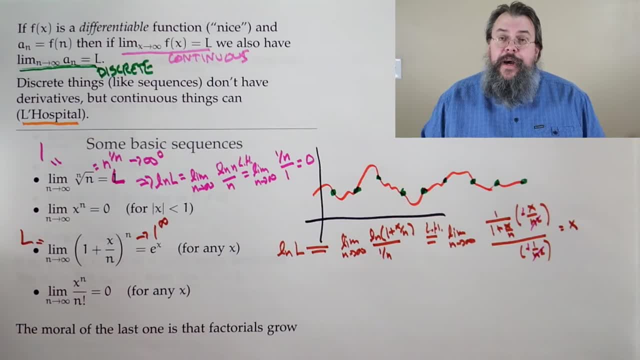 of x to the n over n factorial. Now it might help to remember what n factorial is, because we look at it and say, oh, it's N. you know, because there's an exclamation mark right When you see N factorial. what that? 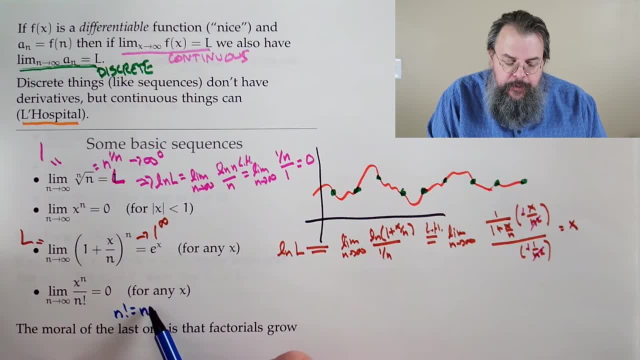 stands for is it just says: start multiplying it and you keep multiplying all the way till you get down to one. So that's what N factorial represents. So the claim is: if you look at X to the power N divided by N factorial and then you let N get bigger, that's going to be getting smaller, and 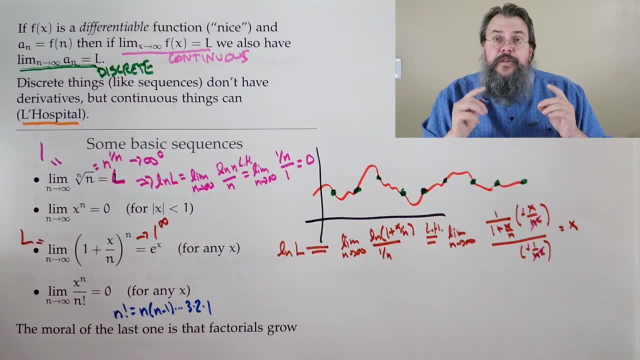 smaller, You might say, okay, well, that's not too surprising, but this is for any X You could choose. X equals a million. a million to the N, That's huge, gigantic numbers And N factorial. sure, they're numbers, but are they big Really, Are they? Well, the answer is yeah, if you let. 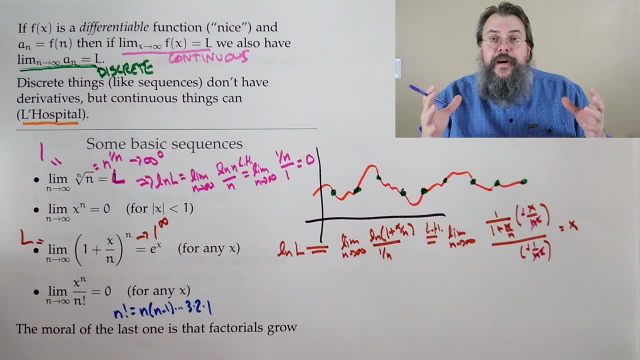 it go If you let it go for a while. I mean sure, small numbers. five: factorial it's 120, not that impressive, but then you get. you know, eight: factorial is 40,000 plus a little bit more. 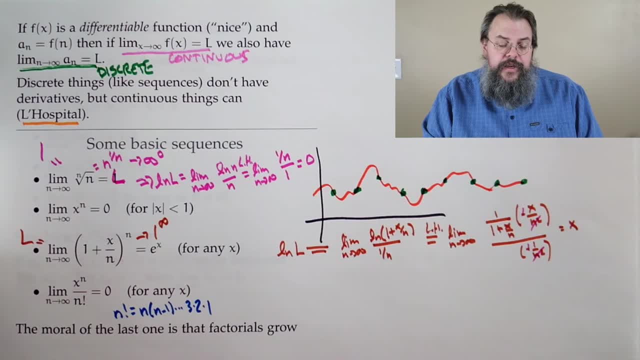 And that's okay. that's a big step up And so it grows quickly. So what's the argument? So here's, I'm going to do a little, a little bit of hand-waving argument here, but enough that we can get a flavor and say, okay. 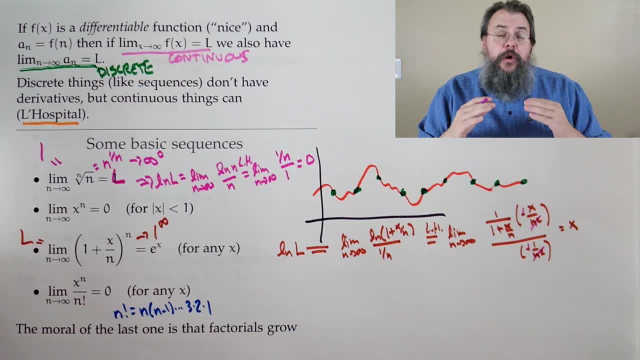 how do we think of X to the N over N factorial? If you think of what N factorial is, what do we see? Well, you have your N times N minus one, times N minus two, down to one, So you have N terms. 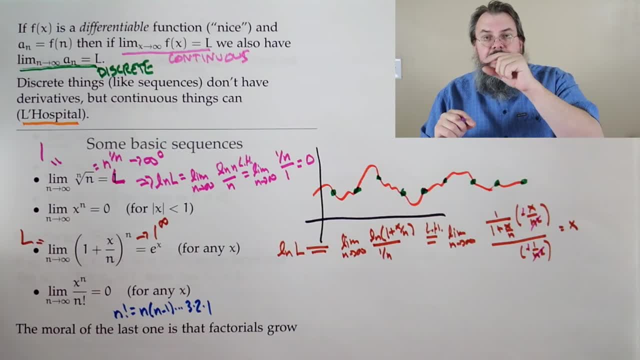 downstairs. Upstairs, you have an X times an X times X, You have X term. sorry, you have N terms upstairs, So we can think of X to the N over N factorial. You have X over N, X over N minus one, X over N minus two, and so forth and so on. 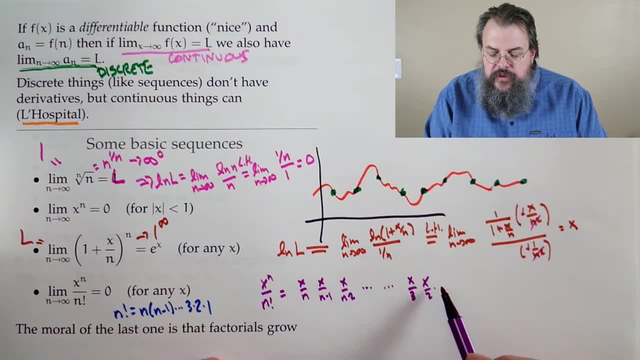 down to, eventually, where you get X over three, X over two and X over one. All right, So that's how we can think of it. Now we're going to let N get big, And here's the key idea. Notice that the 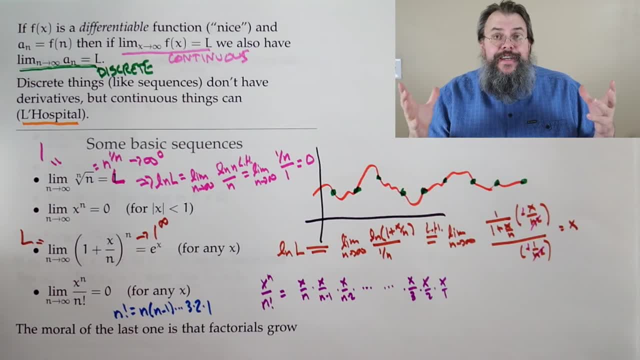 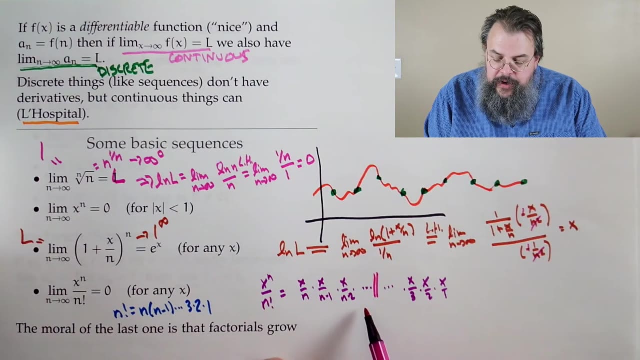 top the X, it's always X, but the bottom gets bigger and bigger. So the key here is an observation that says: look, there's this sort of dividing line where, if I look at all terms over here, X over N is small, It's less than a half. So you might say: 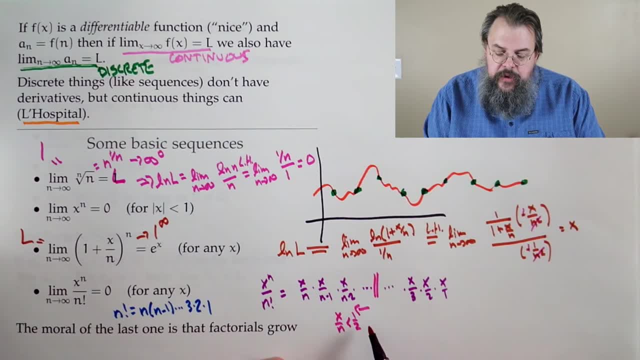 well, when does that happen? Well, that's really says whenever N is larger than two X. So, whenever N is larger than two X, I'm going to look at those terms over here, And I'm going to look at those terms on one side. Then I have, on the other hand- I have these terms over here, Now the key. 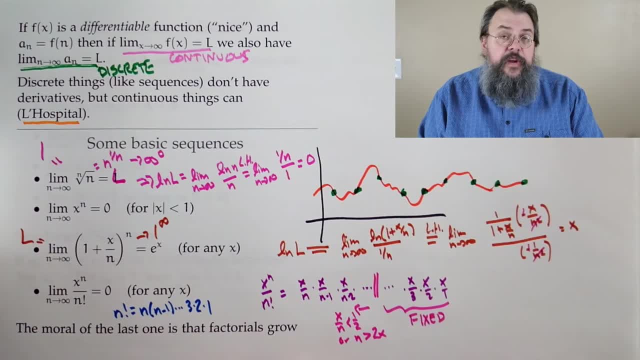 thing about these terms over here is it's fixed. So as N gets large from the dividing line and above, that's going to, you know, there's going to be more and more terms added on this left-hand side. over here It's a fixed value. Nothing's changing. If I have a fixed number then I keep. 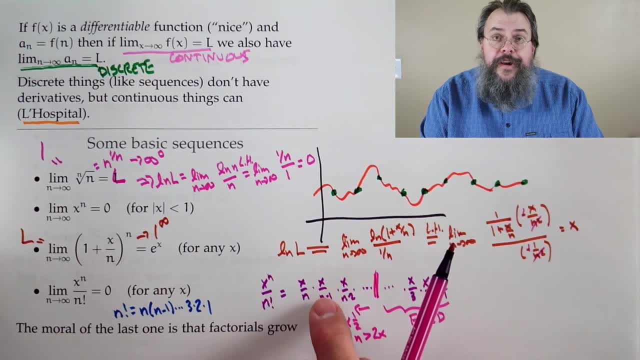 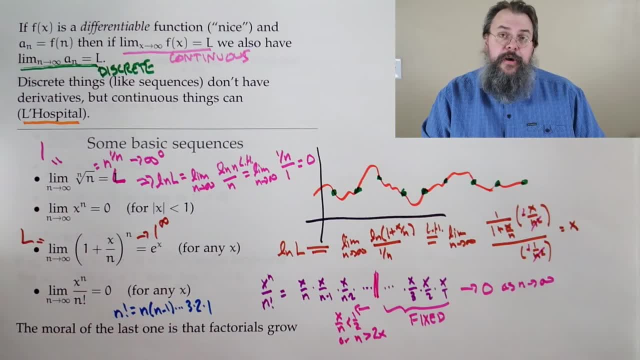 I say a bunch, as many as I need. So it's going to drive it down to be small. So that's the idea. So there's an important moral here That says factorials grow fast. In fact they grow faster than exponentials. So that's the idea. So there's an important moral here That says factorials grow. 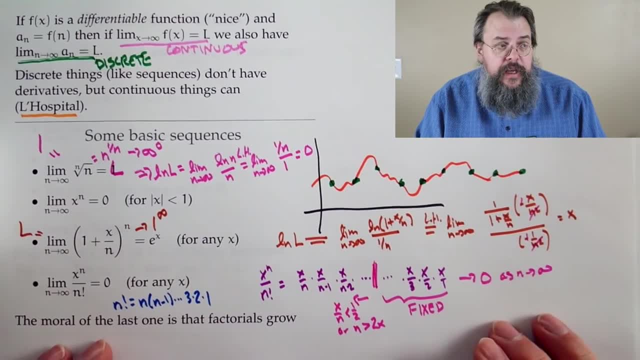 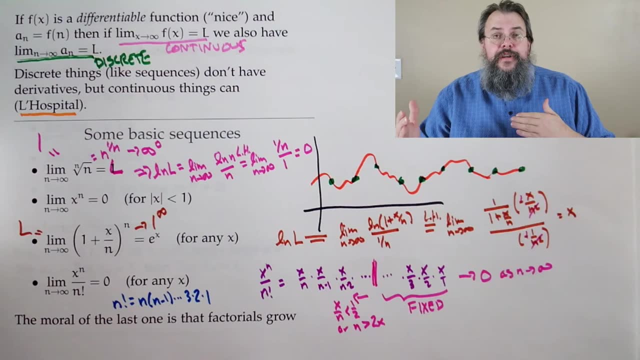 faster than exponentials. Now, one of the things that's going to be very helpful as you go forward is to sort of get an intuition: What's the relative rate at which things grow? In other words, if I want to compare different types of objects and say, well, does this grow faster or? 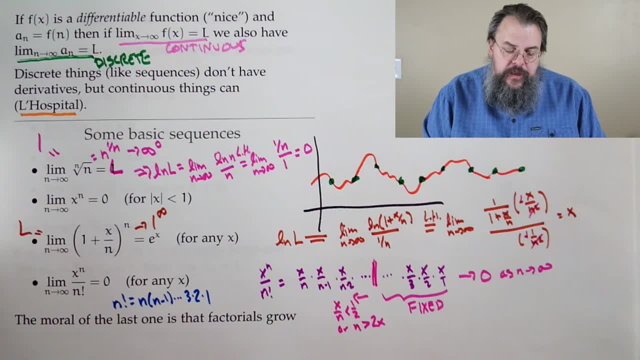 slower. So we'll talk about some really very small, simple hierarchy. So here we go. If you look at a constant, so I'll use C for constant. That's going to be much smaller than so. I'm using two less than signs to say in the long run. 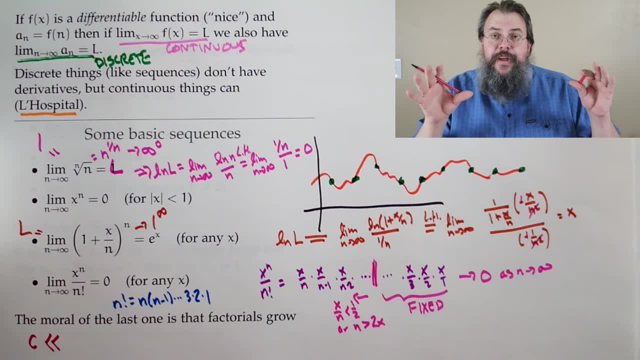 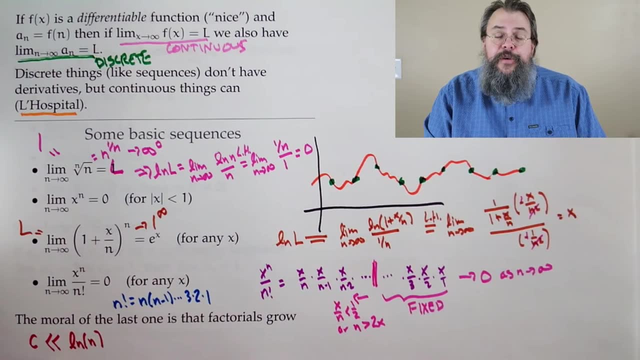 it's very small compared to. So that's what you should think of when you see this notation. That's very small compared to natural log. Natural log will always be the constant, but it might take a while to get past that constant if it's a big constant. 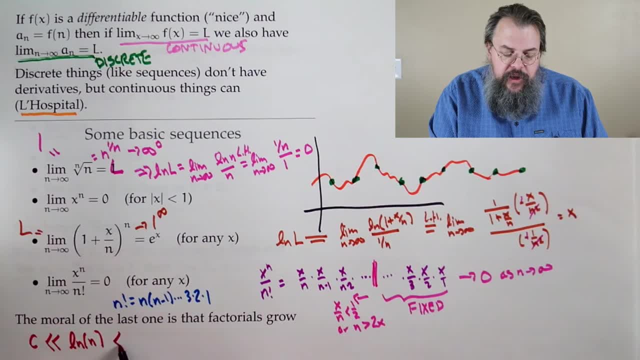 On the other hand, natural log is pretty slow. That's less than n to any power, like you want, and, as long as well, n to any positive power. so n to the point: zero, zero, zero, zero. one eventually beats natural log. It'll always happen that way. On the other hand, n to any power. 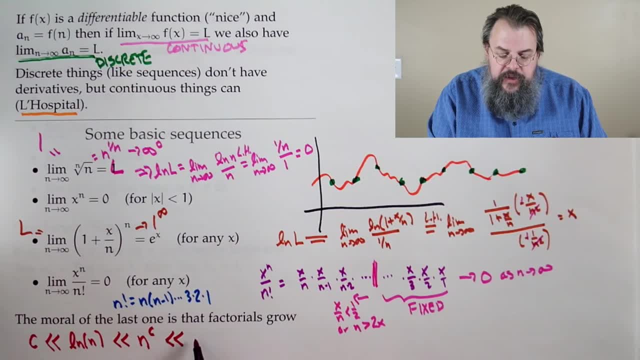 well, that's polynomial That always loses out to exponential. So here I should say C is greater than one. Here this is: C is greater than zero. I probably shouldn't use the same symbol. Okay, I'm switching it. This is now a d. 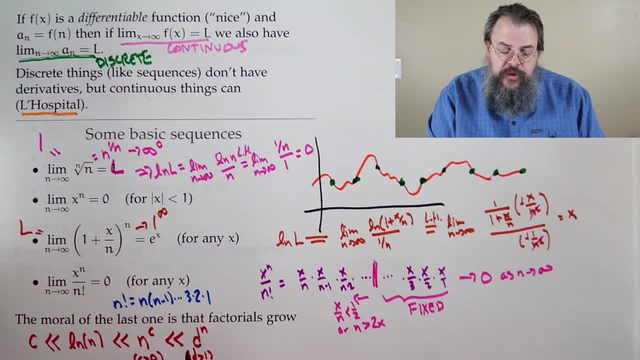 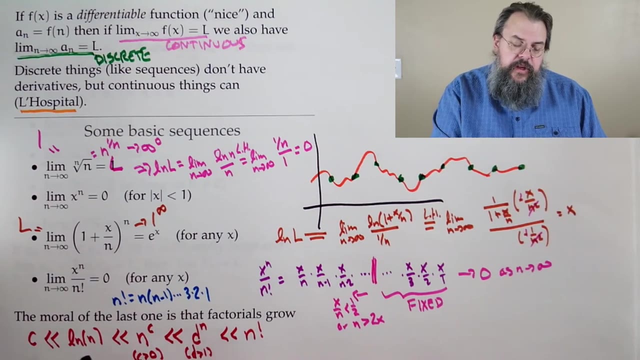 All right. So polynomials lose to exponentials. Exponentials we just said they lose to factorials. So when you're doing a comparison, just remember: polynomials lose to exponentials, Exponentials lose to factorials. 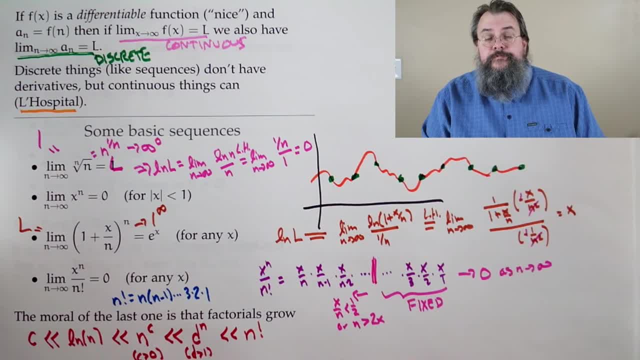 Logs rarely slow, but at least they're bigger than constants. So all right, I will from time to time point out and say, hey, it's nice to know which things are growing faster. Now one last small idea. 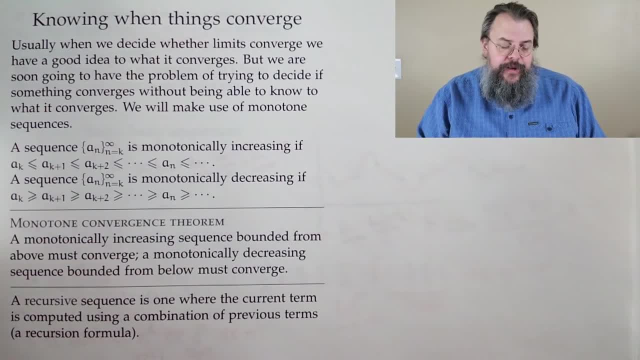 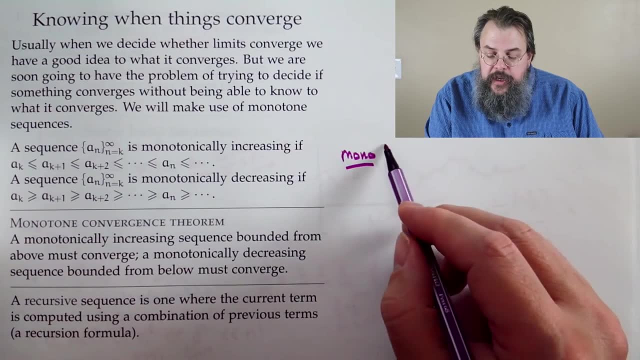 And this is monotonic sequences. Now, when you think of monotonic, you might say: okay, what does that mean? Well, mono means one, and tonic is a type of drink, So this is something that requires one drink to understand. 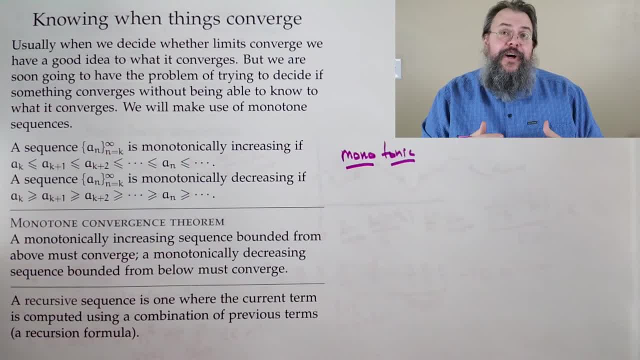 No, no, no, no. That's not what monotonic means. Monotonic just means one type of behavior And in particular, we can talk about things like increasing and decreasing. So if we're talking monotonically, increasing, the picture says: when you look at your terms. 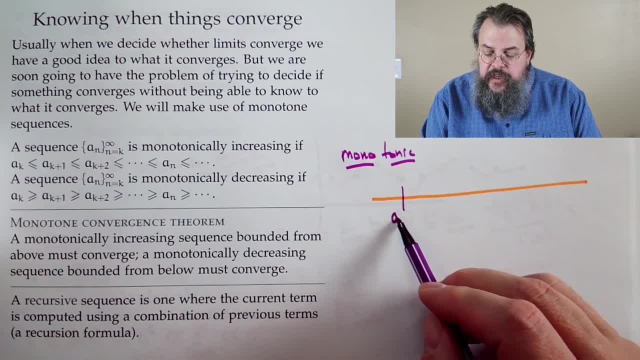 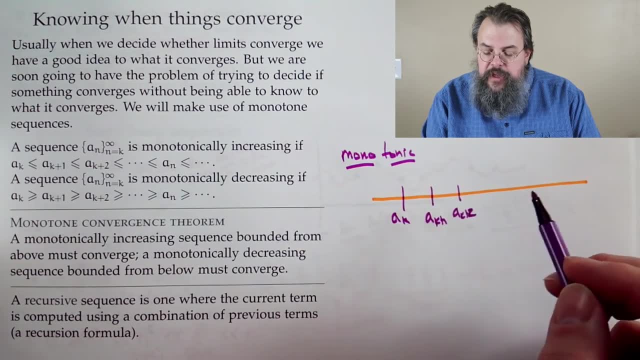 they only go in one direction. So here's like the a k, then the next term a k plus one, and then the next term a k plus two. Now they might be spaced further apart, They might be spaced closer together. 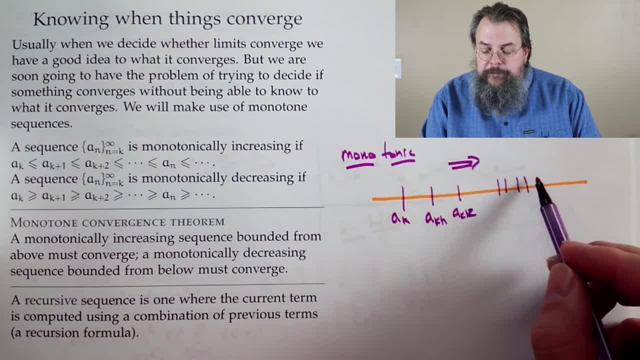 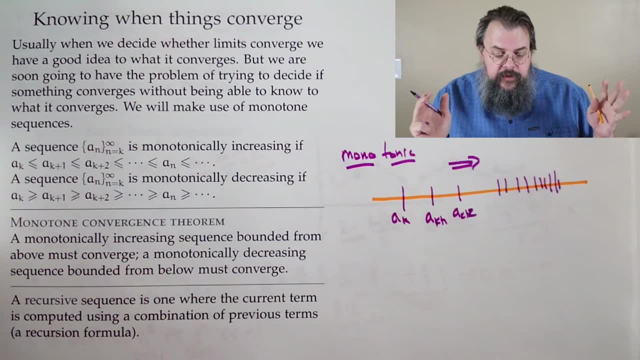 But they're always, they're always sort of going in one way. So that's monotonic. And that's increasing if you go one way, decreasing if you go the other way. Okay, so that's the idea. There's this nice result that says: if you are monotonic, 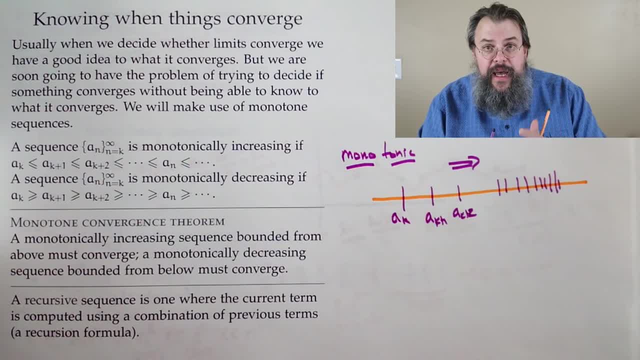 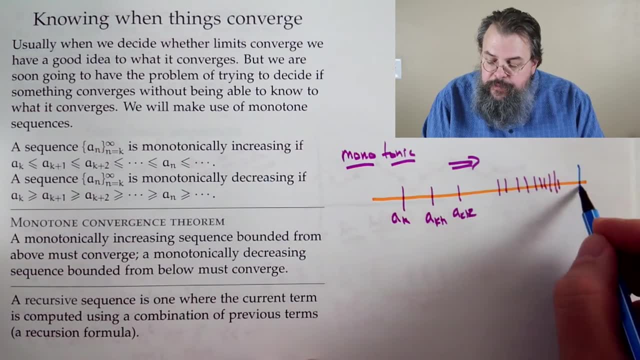 so you have one type of behavior and you're bounded. So what does that say? Well, to say that you're bounded says: look, you don't go past the third threshold. This is your bound, This is a you cannot go past here. 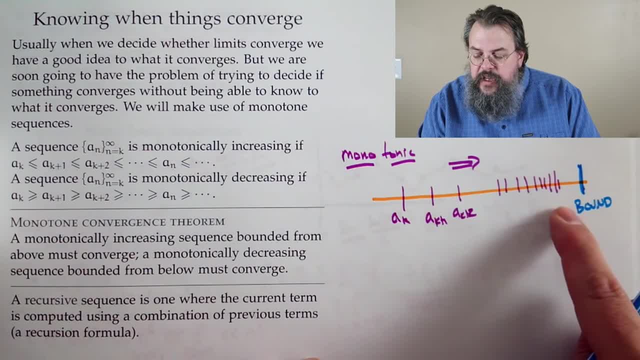 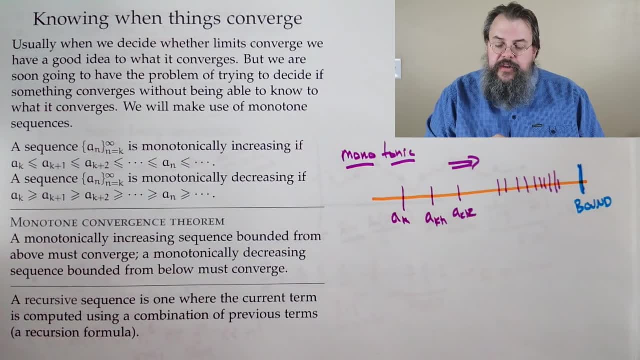 So you can go up, but you can't go past. You can get as close as you want and you don't even get close to it. We're not even claiming it's the ideal bound, that it's the best bound. It's just saying there's some bound where it says: look, you'll never get past that point. 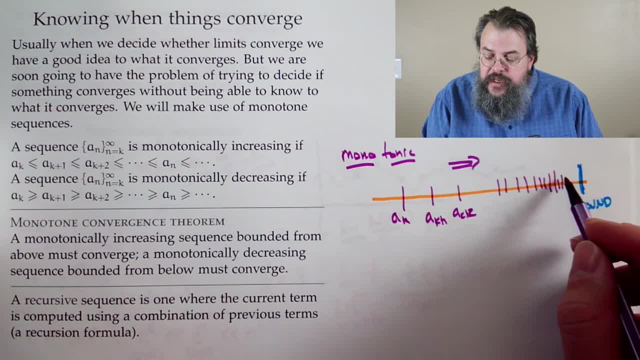 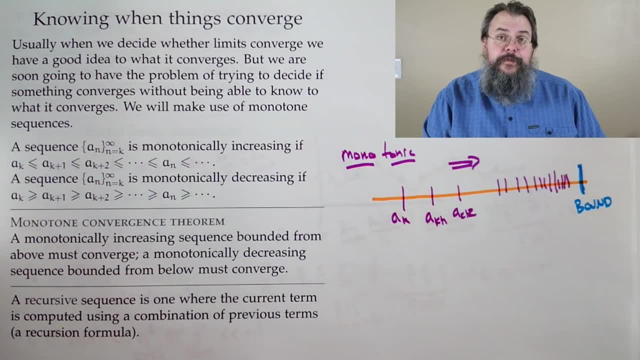 Then what's the conclusion? The conclusion is: there has to be some place where you converge. So there's some point, a limit point that you converge. Now, why is this amazing? Well, this is amazing because it says: wait a second, you may not know what it converges to. 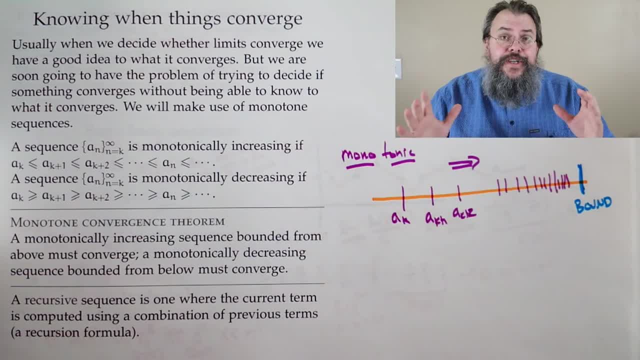 Because our conclusion is just: it converges. We're not making any claim that says, oh, it converges to this value. We just say we know it converges to something. So it's this wonderful idea in mathematics that we say, hey, we know something happens. 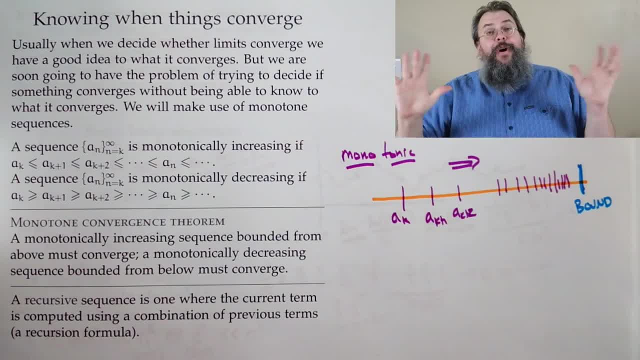 You might say: oh fantastic, what is it? We don't know what it actually is. Okay, We don't know what it is, We just know it happens And it's a fun idea. We won't make much use of that, but I just want to say that there does exist this tool. 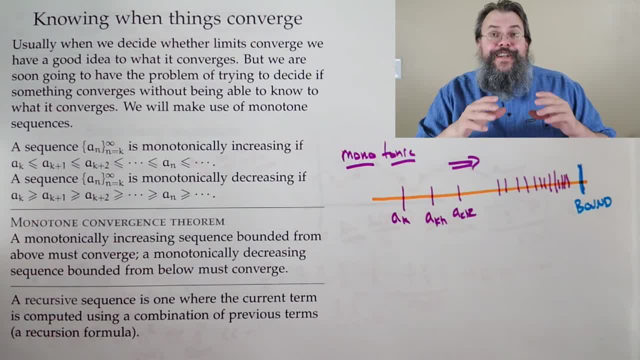 And if you want to know more about it, keep going, take more classes. Last thing to mention for today is you will from time to time see something which are called recursive sequences. Now, some people are fairly familiar with a really special case known as the Fibonacci numbers. 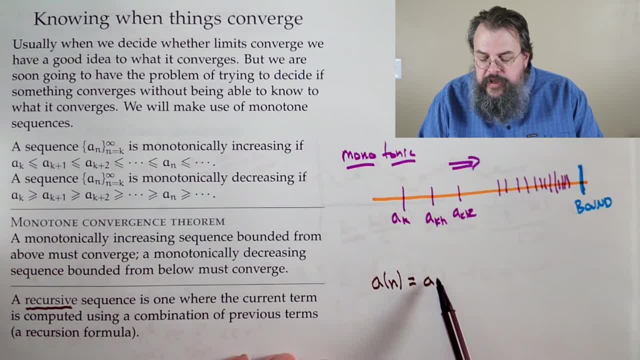 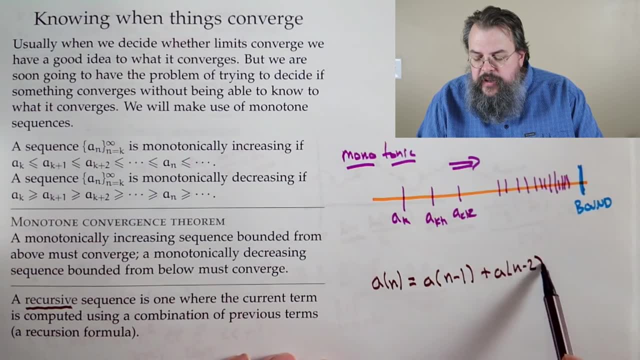 And if you see that this will be sort of a proof by rather- excuse me, a definition by example. So the Fibonacci numbers say what: Add the two previous numbers to get our next number. So when we talk about recursive sequences, it just really says: oh, if I want to know what my current value is. 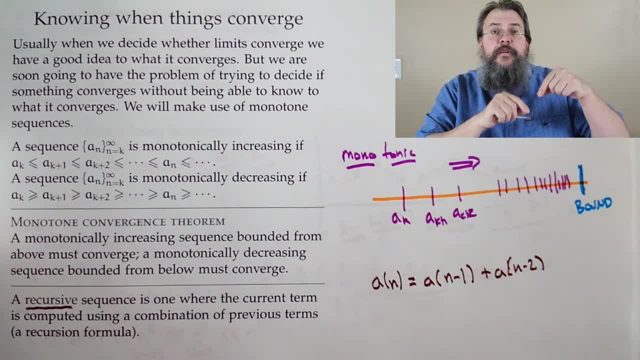 look at the values that came before and use them in some way. So it sort of builds on things in some nice iterative way. It builds on some nice iterative process. A lot of natural problems are recursive. It says, hey, if I want to understand what the current thing is, I should look at the previous terms. 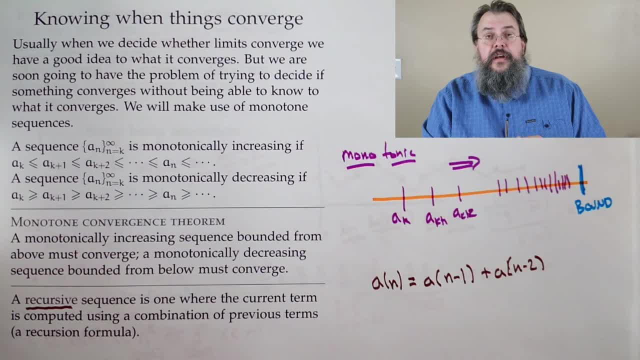 because that informs my current behavior. It also shows up in certain applications when you get to, say, differential equations. One of the ways that we can solve problems are we can look at what we call series solutions. We'll talk about that later on. 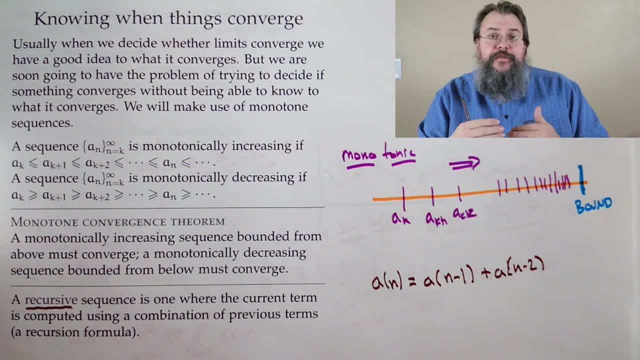 But hey, it builds off of this notion of saying: look what's the next term, I can figure out by saying what's the previous terms, And so all right. so that's what recursive is, And we'll do some examples.